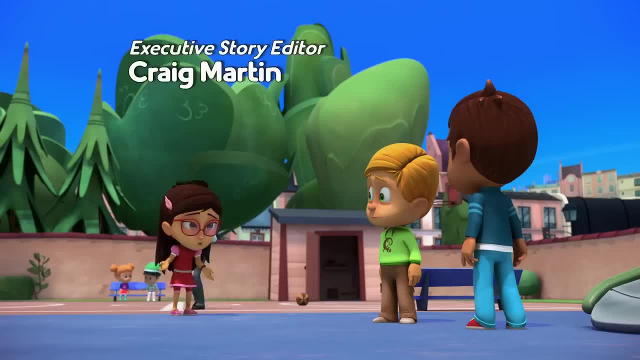 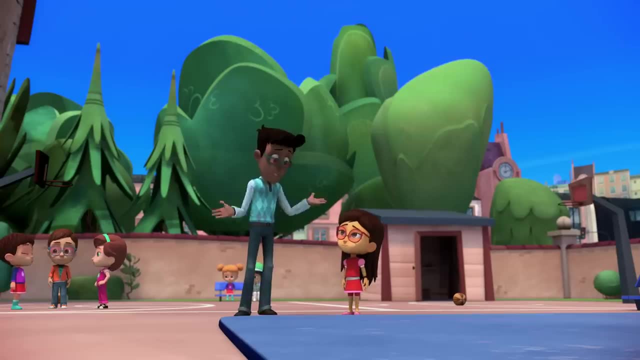 Can you teach me? Sure, but the forwards roll was supposed to be my thing. Can you show me how to do a cartwheel? I would, but I need to find the gym mats. The shed is completely empty. Really, That's strange. 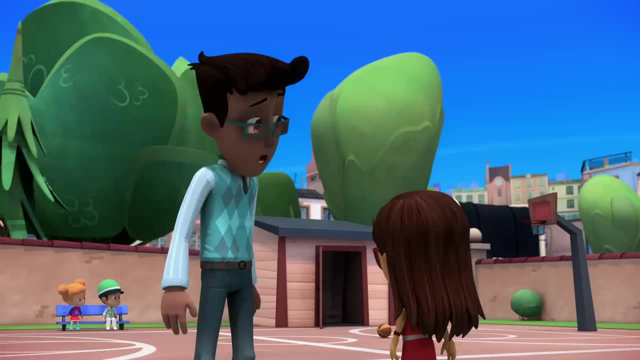 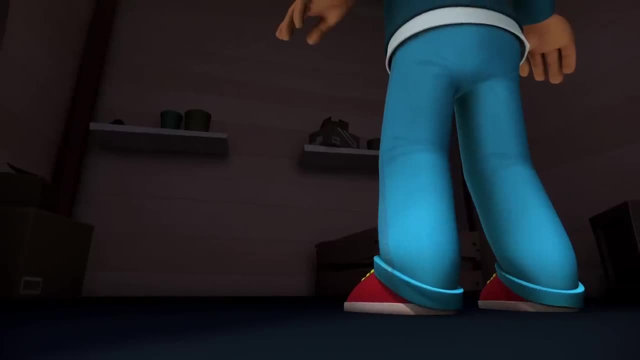 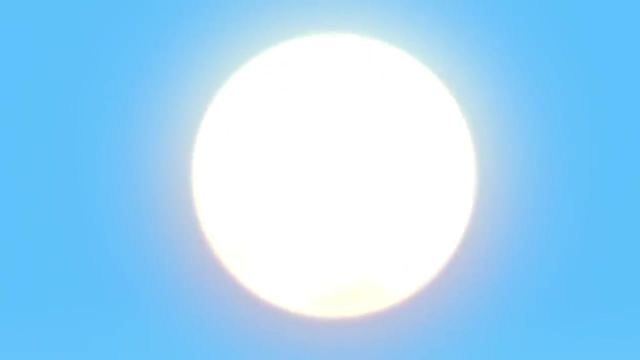 It sure is, especially since all the paint brushes and balls are missing too. Something really strange is going on today. This sounds like a job for us, PJ Masks. we're on our way Into the night to save the day Night in the city. 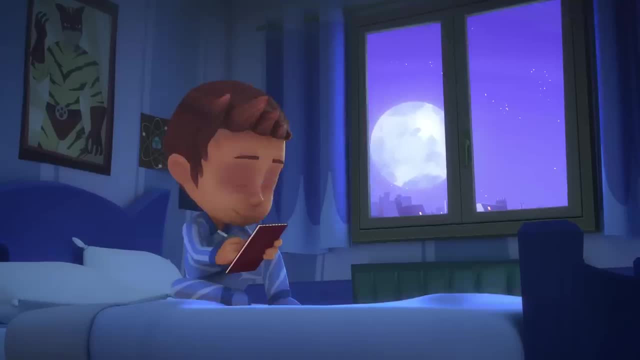 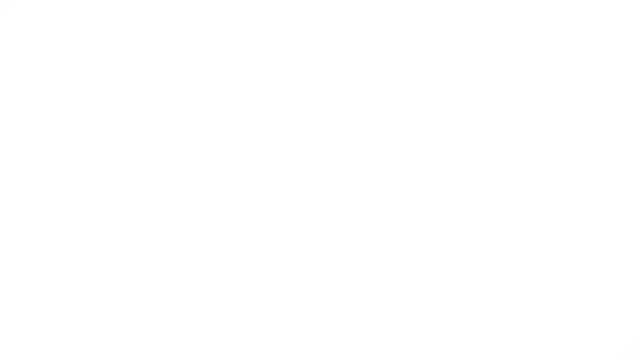 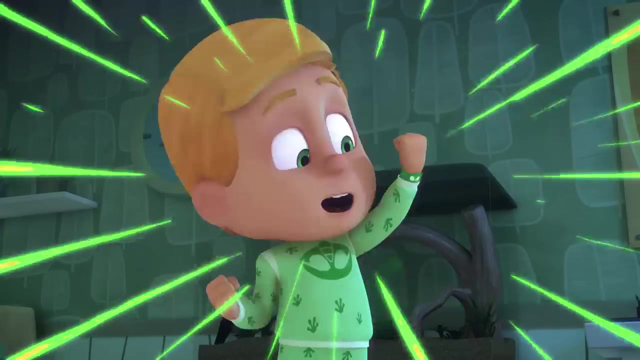 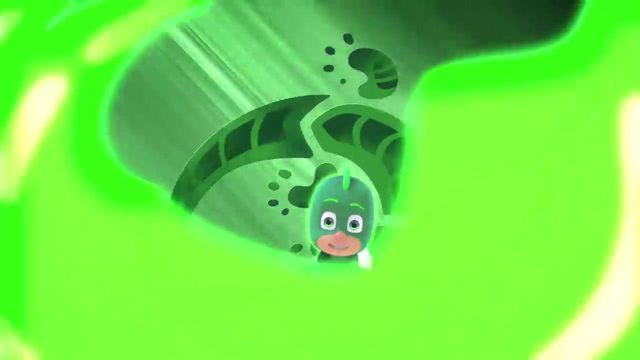 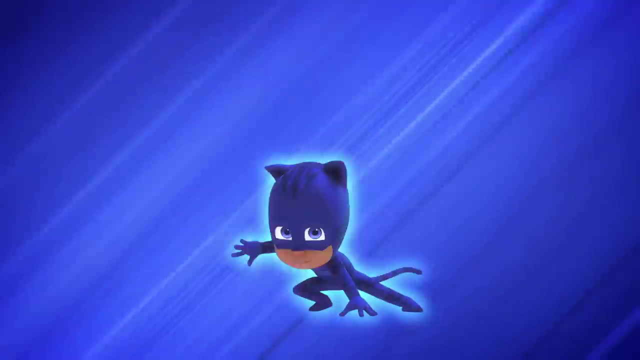 And a brave band of heroes is ready to face fiendish villains to stop them messing with your day. Amaya becomes Owlette- Yeah. Greg becomes Kick him, Yeah. Connor becomes Catboy: Yeah, Yeah, Yeah. 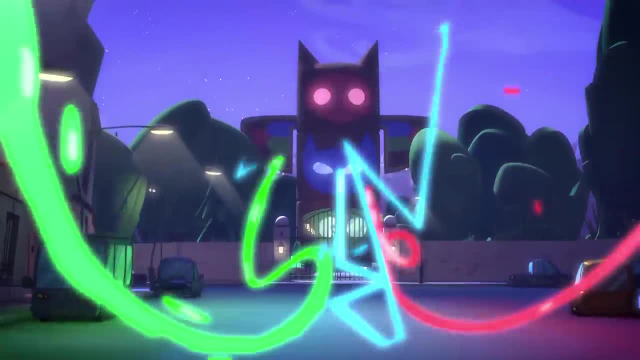 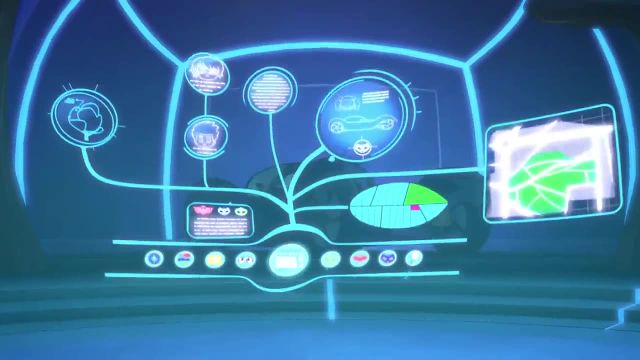 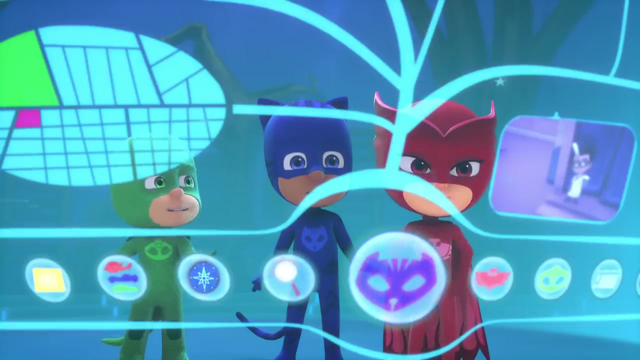 Yeah, Yeah, Yeah Yeah, The PJ Masks. We should start by checking the school for villains like… Romeo. But why is he just standing there like that? Who knows? We have to stop him before he makes anything else disappear. 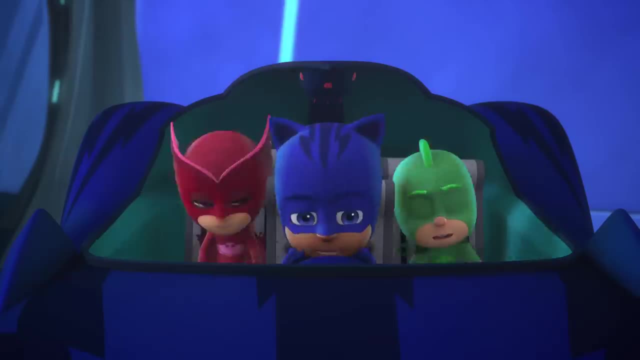 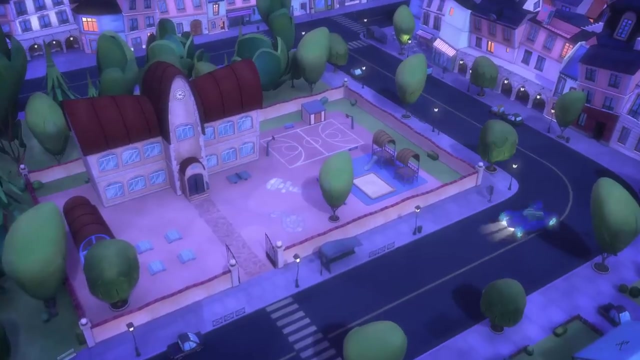 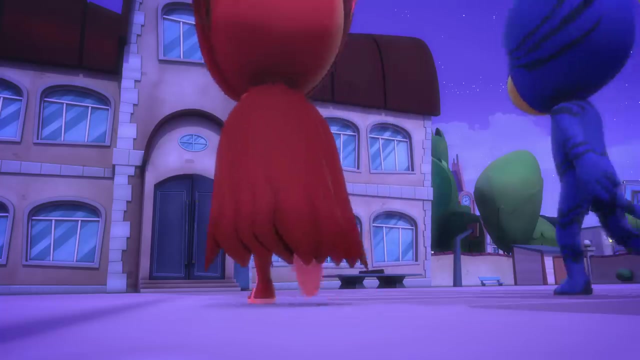 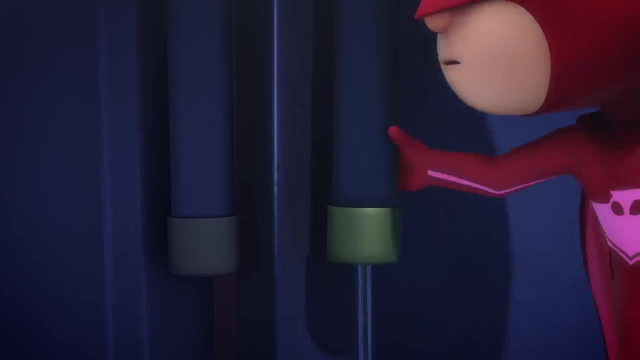 To the cat car. To the Cat Car: Where's Romeo? He must have gone inside. Let's check it out. Be careful. I don't know what he's up to, but it's never good. Romeo, we know you're in here. 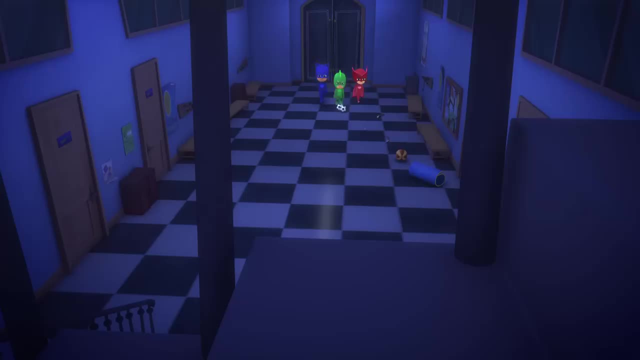 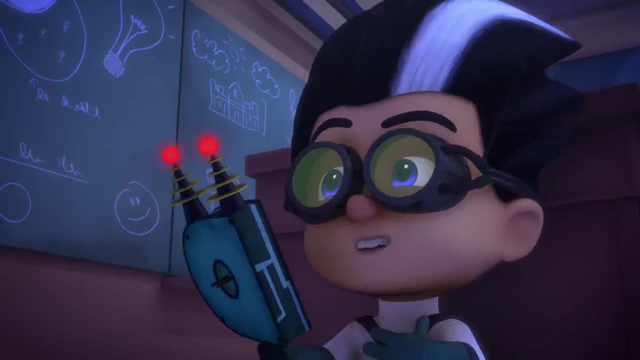 Why don't you save us all some time and give up? If we follow this trail of missing stuff, it should lead right to Romeo. This plan is brilliant. Well, all my plans are brilliant, but especially this one. Once the PJ Masks trigger my trap. 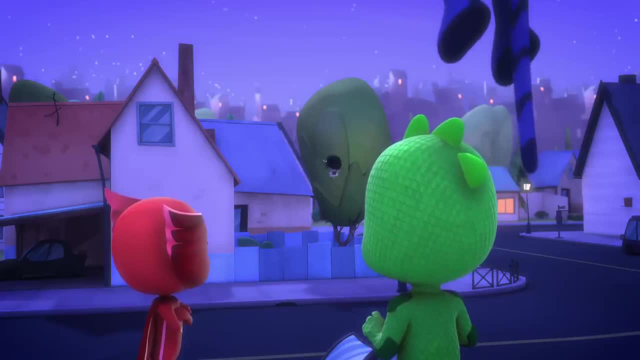 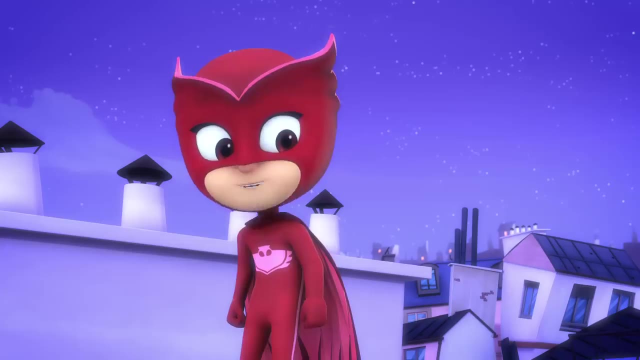 Ooh, Ooh, You guys going to chase me, or what? Whoa, Come on PJ Masks. Let's find Romeo. Why don't I fly and you two look from the ground? But we can see so much further from up here. 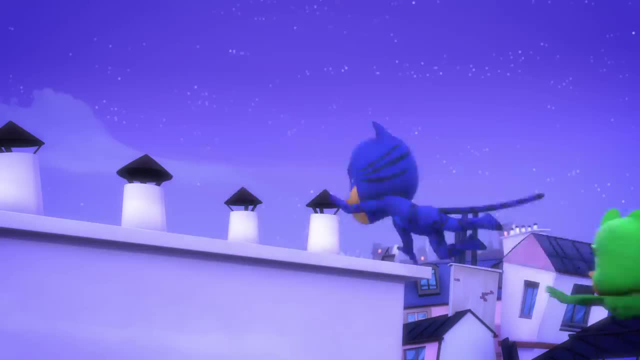 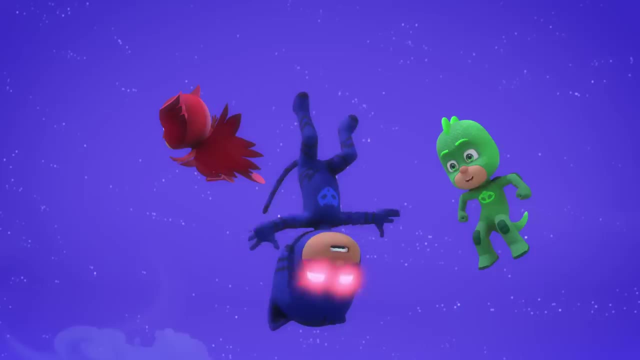 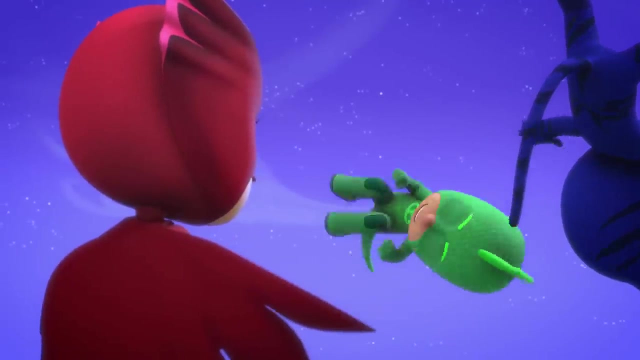 Plus, this is way more fun. Yeah, I can't see Romeo anywhere. Are you using owl eyes? Yeah, but I call it cat eyes. You have my owl eyes? Owl eyes power too? Ooh, let me try. 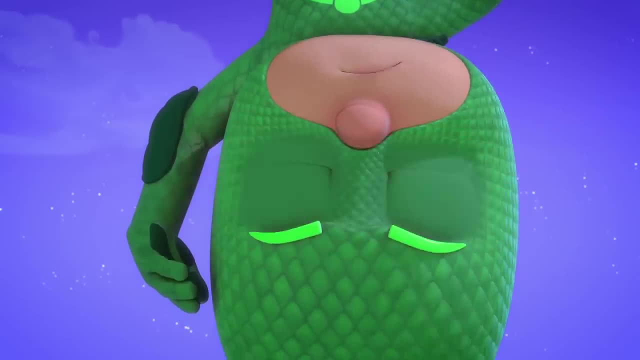 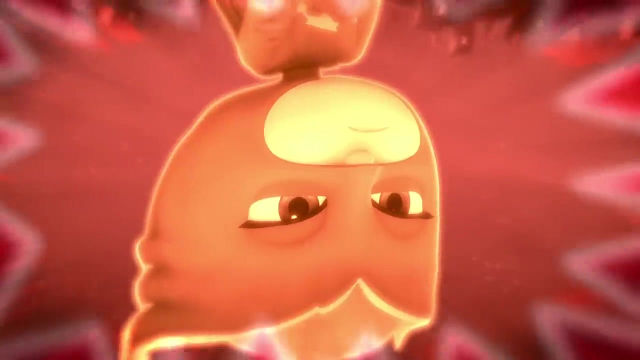 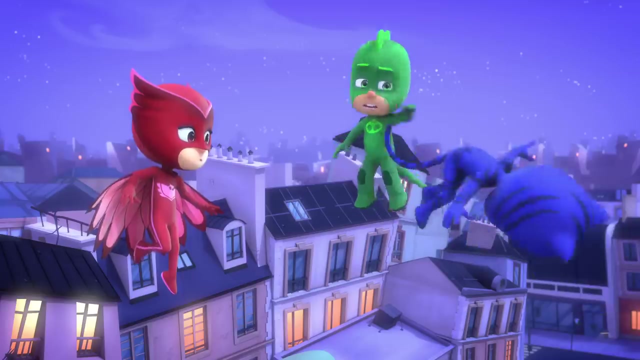 Gecko vision. Oh, I see Romeo. Nope, I think I got him. Nope, There he is. Oops, How do you use owl eyes to see things super close up? Ah, Hey, I just did a flip. I think I see Romeo. 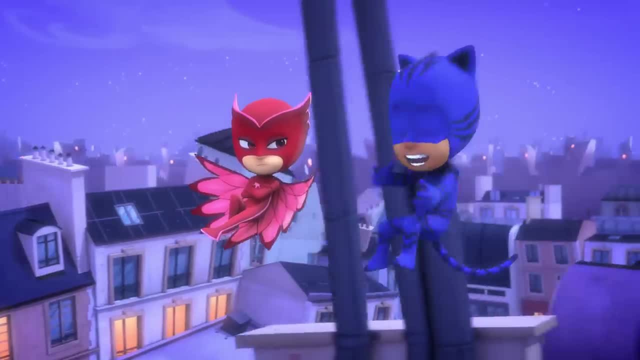 Over there. Hey, you're not doing it right, Are you? OK, Yeah, but I'm stuck. Guys, he's getting away. One more pull and you're capes free There. Come on, Let's get him now. 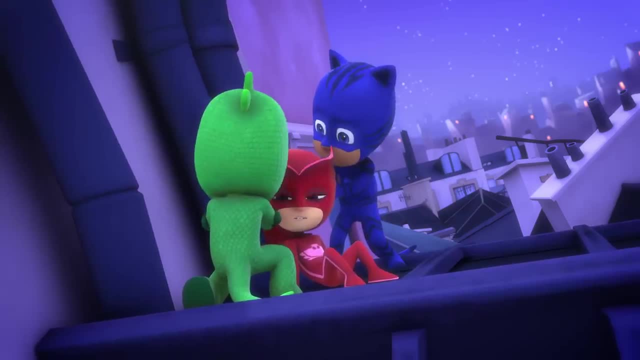 Whoa, Flying is my thing. Why don't you land? Because flying is awesome. Besides, if we all fly, we can catch Romeo faster. Maybe you can show us some moves, Like how to stop and do a loop-do it. 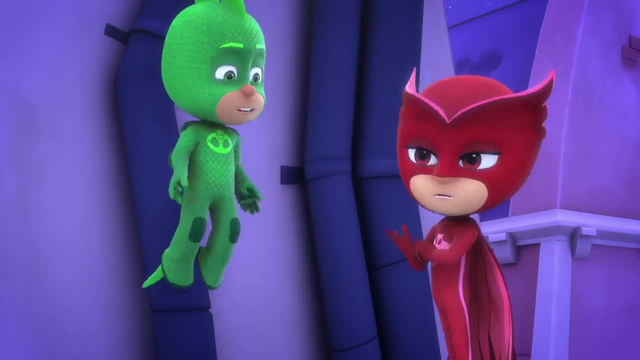 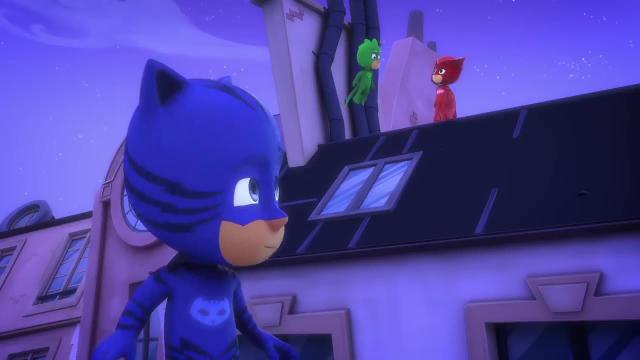 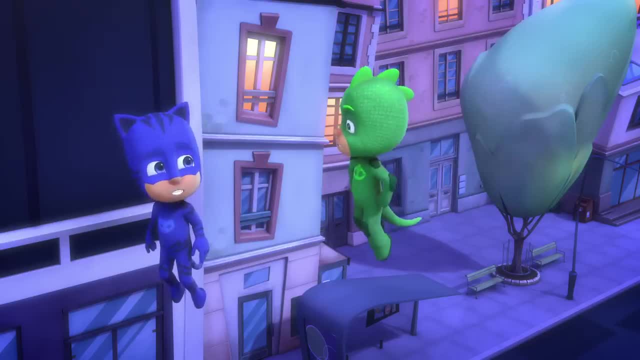 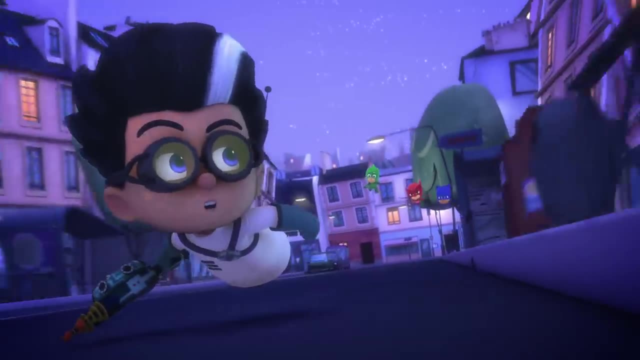 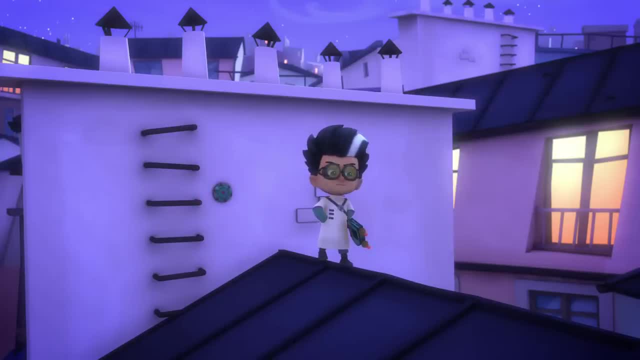 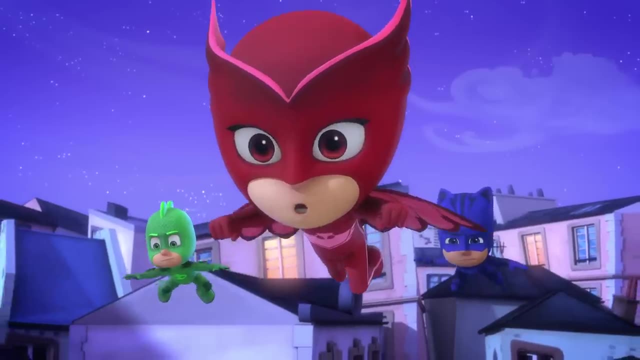 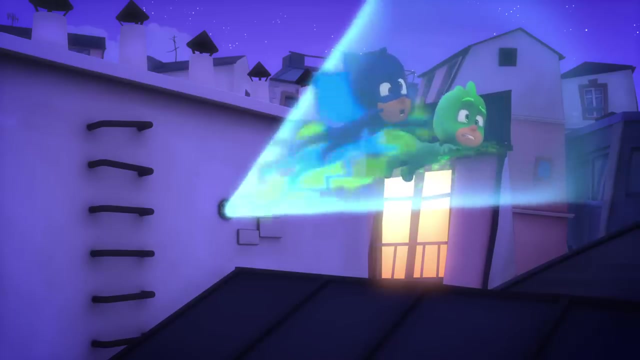 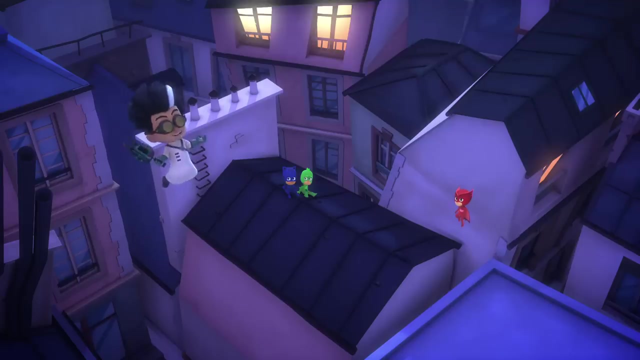 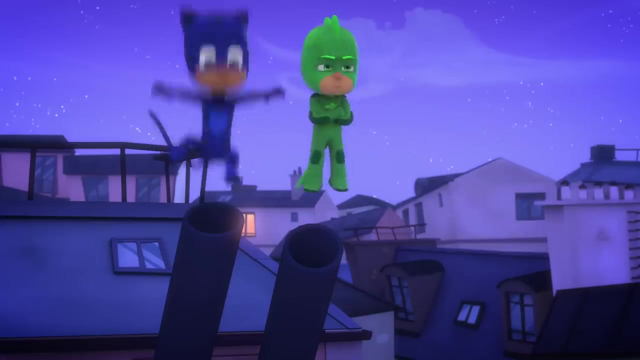 74!, 78! score. knot, knot, Whoa With a由. Watch this, friends. Ha ha ha. Super Catch Thief. Ha ha, Gecko Camouflage. What? Now that I've copied all your powers, nothing can stop me from taking over the world. 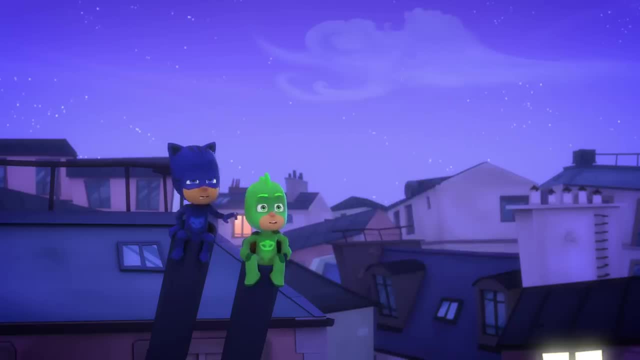 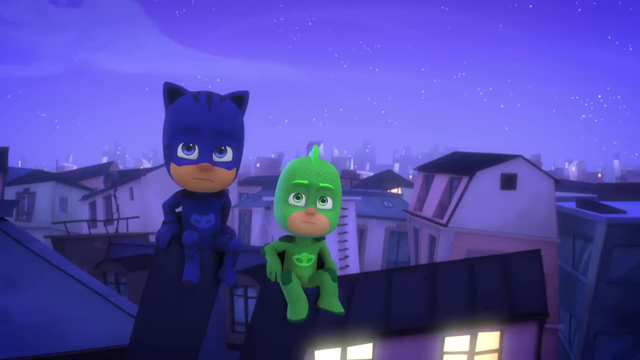 Romeo, you won't get away with this. I already did. With your powers, combined with my genius, I'm unstoppable. So long, PJ Pest. This is all my fault If I hadn't been so upset about you guys getting my flying powers. 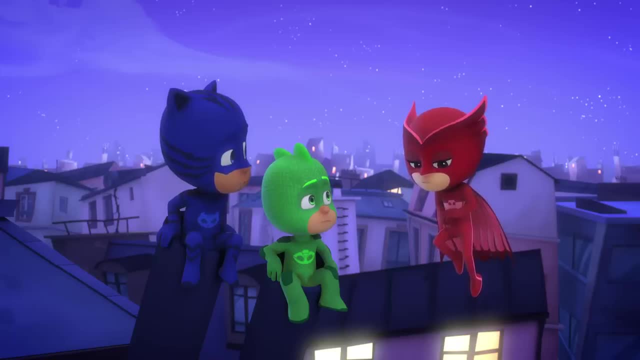 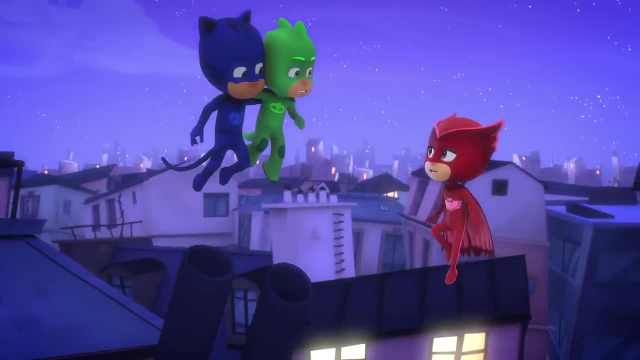 we would have already stopped Romeo. That's okay, Owlette, And we're sorry too. We got carried away using your powers. Now that Romeo has all of our powers, it's going to take all of us working together to stop him. 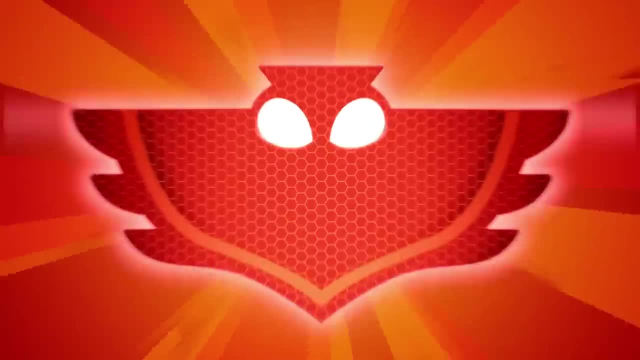 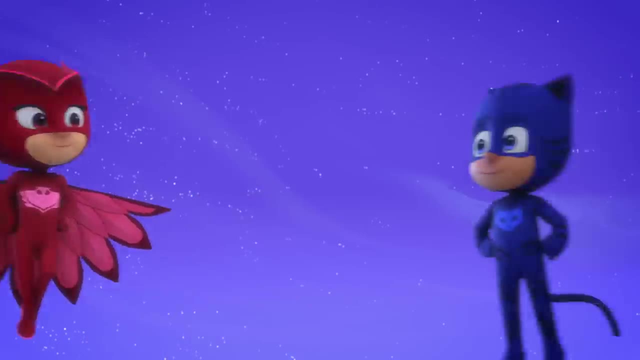 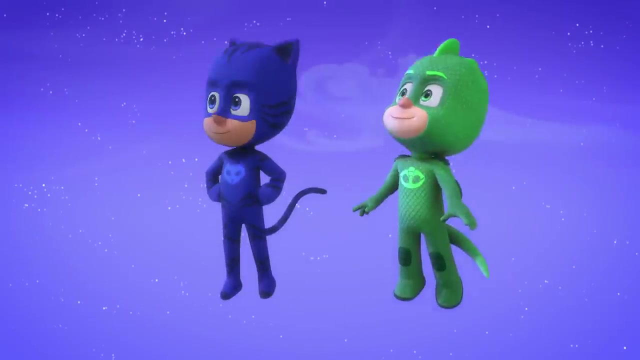 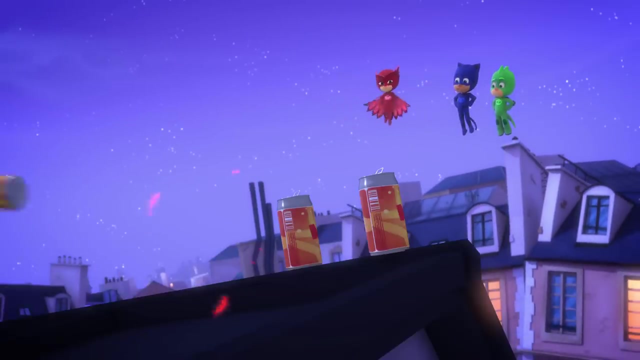 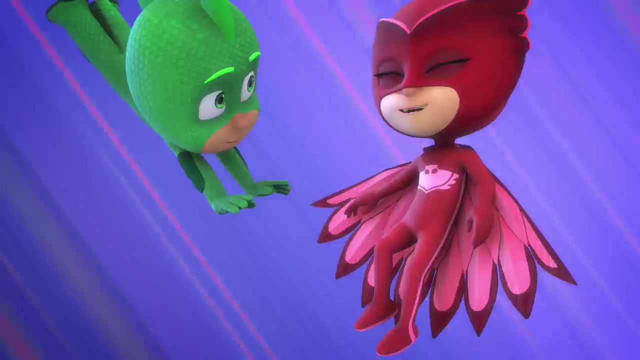 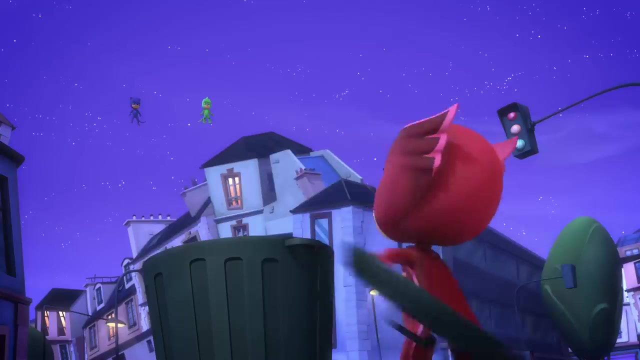 Right, But first let me show you some tricks. Let's see if I can get the. Oh, I got a bit of luck there. I think that's it. Nice pass, Thanks, Hey guys. Catch Woo, Woo-woo. 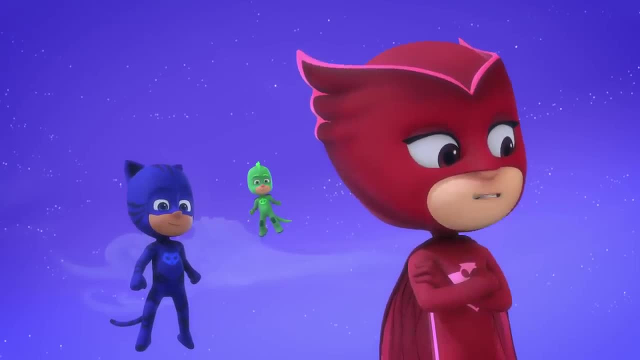 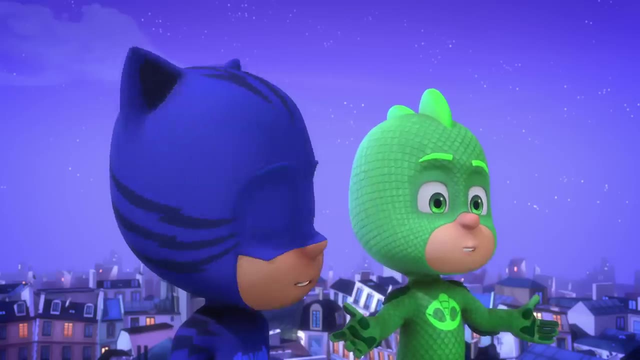 This is pretty cool. I was so worried you were using my powers that I didn't notice how much fun it is sharing them with you. Thanks for helping us learn to fly. This is a blast, And it's even more fun than I imagined. 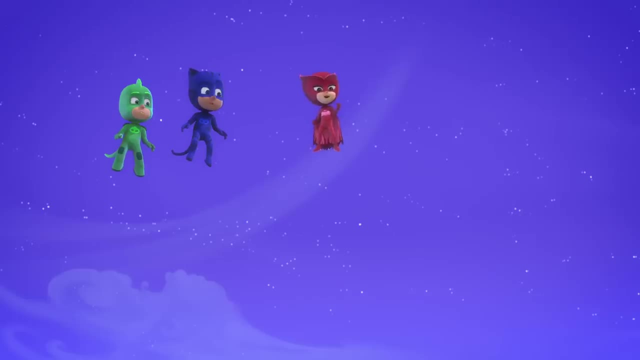 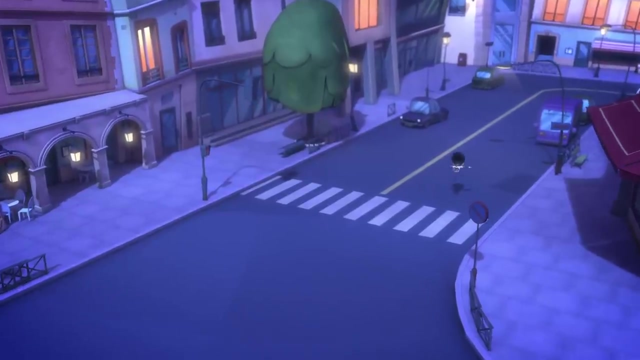 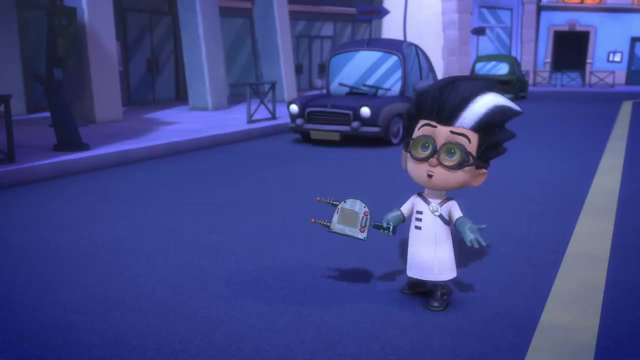 Look, There's Romeo. It's time to be a hero. Woo, Woo-hoo-hoo-hoo Ha. These powers are incredible. Romeo, you're not keeping our powers any longer. What are you gonna do? Break my PJ? power copier. 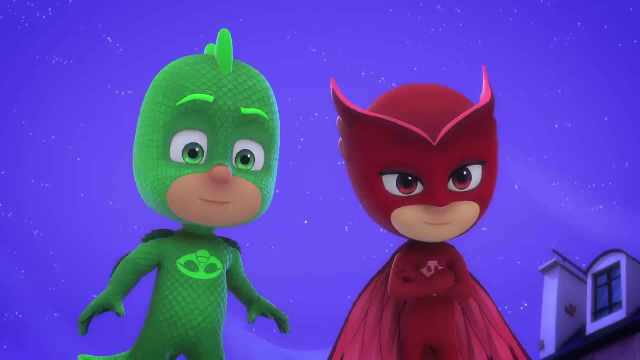 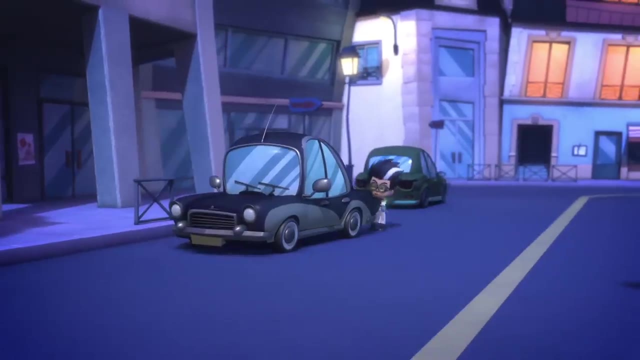 that took me a really, really long time to build, so it releases your powers. Sounds like a good idea to me. Oops, That would do it actually, But first you'll have to deal with my super gecko muscles. Remember everyone, follow my lead. 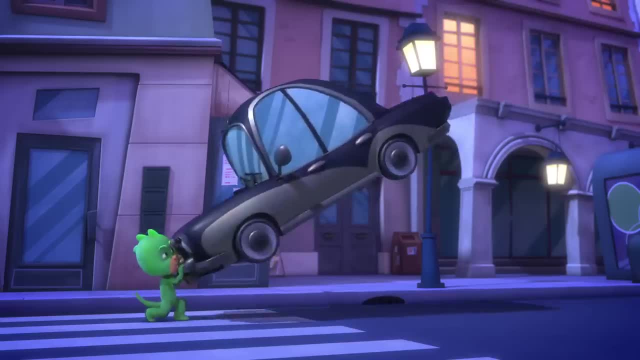 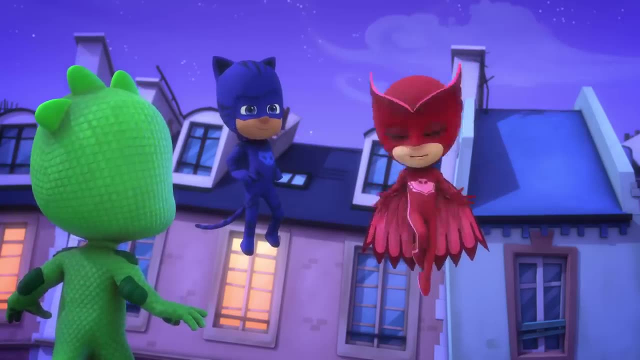 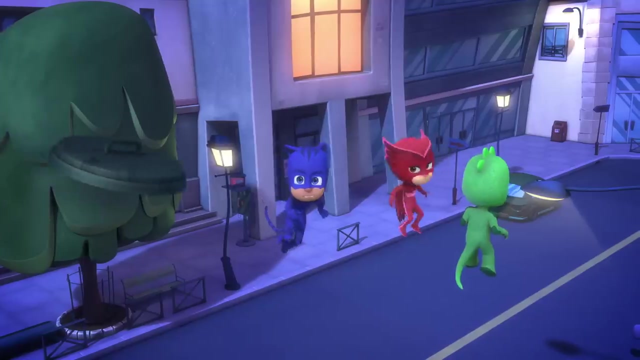 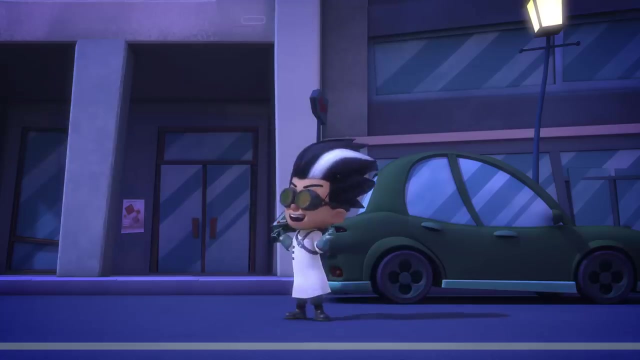 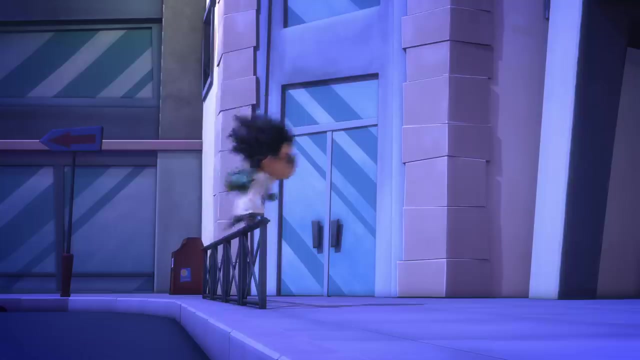 Up Now, Ah. Super Lizard Brick. You heard, Romeo? All we have to do is get that machine Now right. Outlet Ha-ha. Super Cushy Ah, Now surround him. Super Cush Jump Ah. 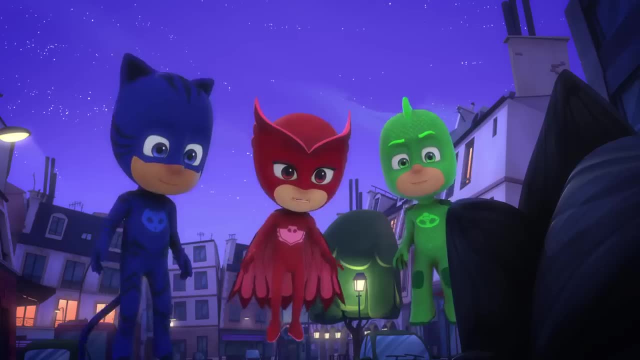 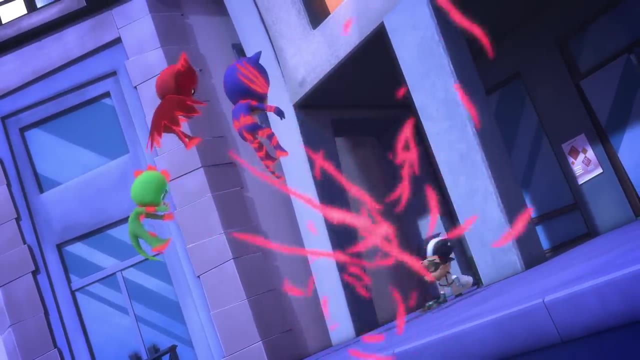 Ah, Ah Ah. Everyone, use your super owl wings. He'll blow the power copier right out of his hands. Owl wings win. Whoa, It's working. Flap harder. Ah Yeah, Super, Cush me Go. 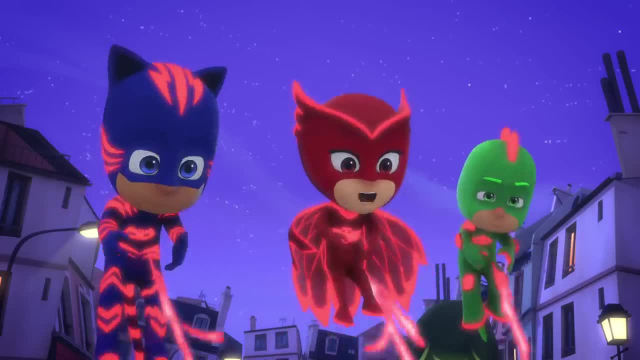 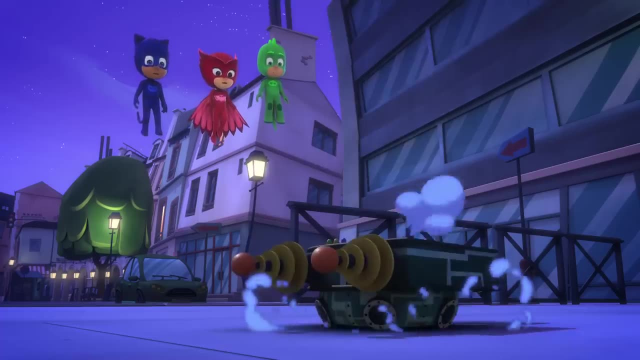 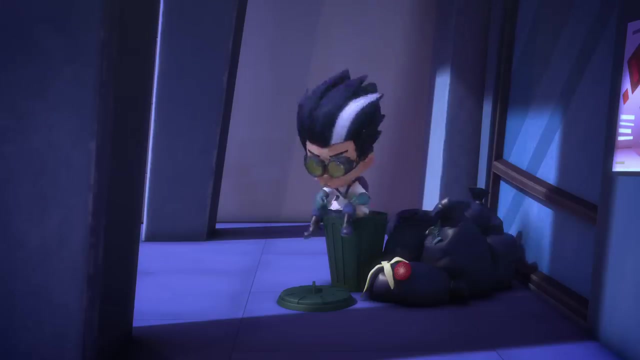 Ah, Super Lizard Grip. Ah, Just a little harder. Ah, Ah, Ah, Ah, Ah Ah, SMASH, All right, help, Gotcha Great Woo. You got me this time PJ Masks, But I don't need your puny powers to take over the world. 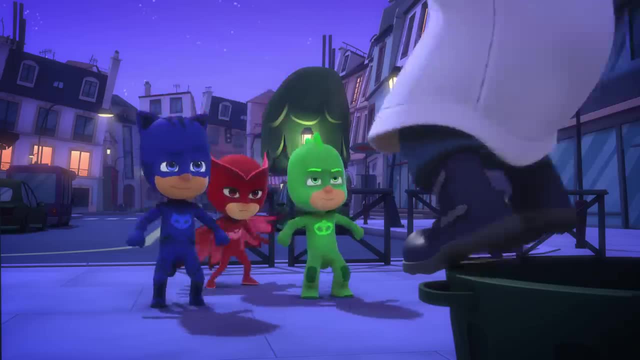 You'll see So long, Romeo. NEXT TIME ON THE UNIVERSAL Del Everest. Now let's put all of the stolen stuff back in the school shed- PJ Masks. I'll shout: hooray, NEXT TIME ON THE UNIVERSAL, Because in that night we save the day. 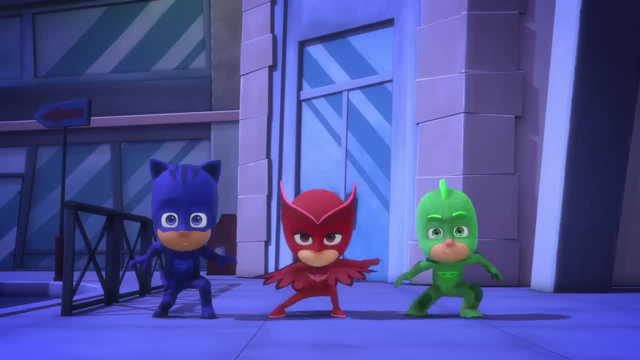 recruits are stove attendants. Video clip here: ESS, PlayStation US AND use your friendly horns while we see. child mask, because they're made of sun-étais R. playground of speed, Because in that night we save the day. CAMERAS ECON2. 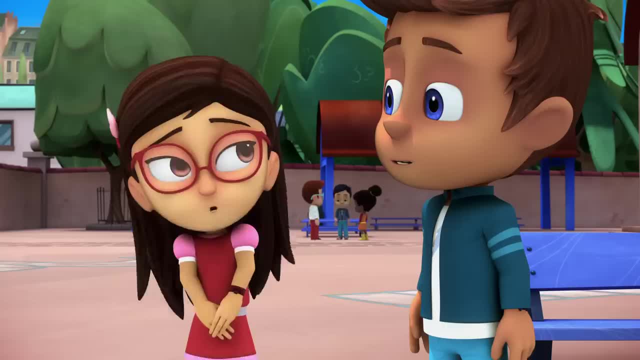 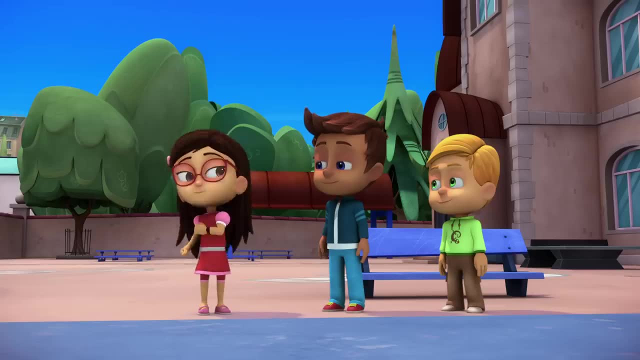 SE advertisement. Hey guys. Um, Connor, do you want to do the Ford's roll again? Sure, I mean, if that's okay with you. Of course, The Ford's roll isn't just my thing And it'll be more fun if we all do it together. 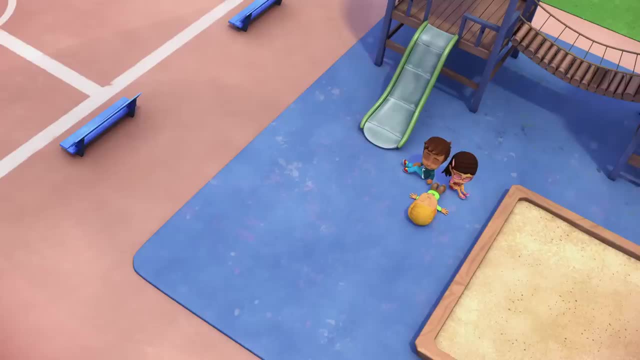 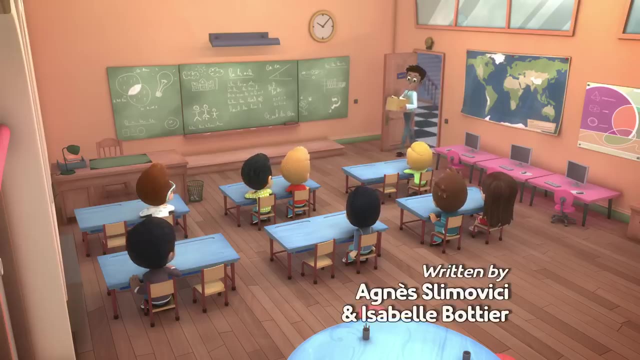 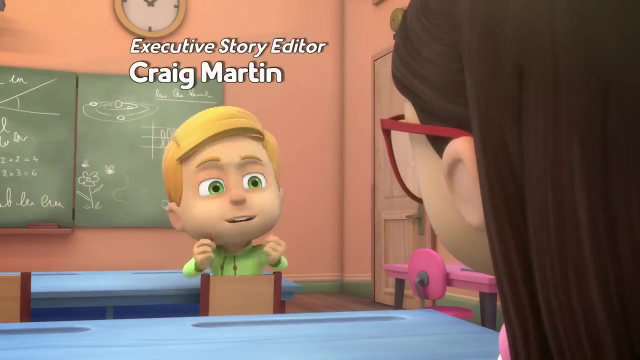 Oops, My turn, Oops, Gekko. and the Mayhem at the Museum. Hi kids, Is everyone ready to build their model rocket? Yay, I'm going to make the best rocket ever. It's going to have lasers and boosters. 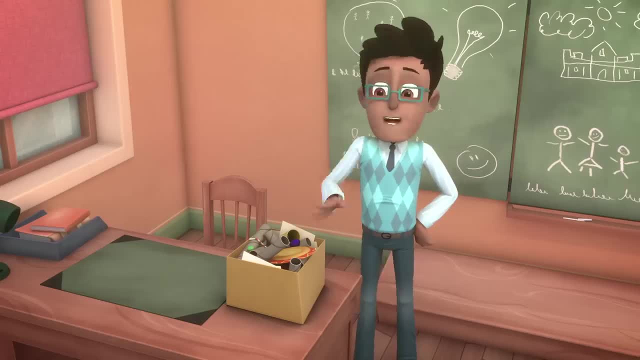 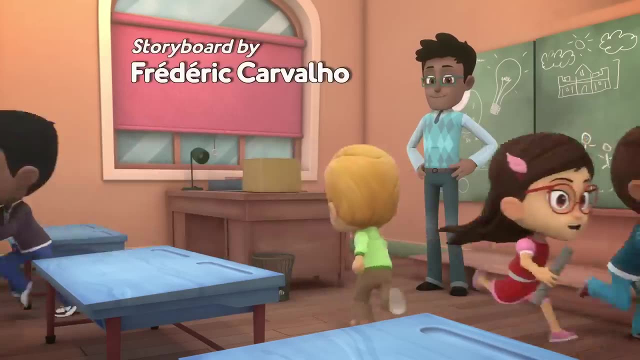 and it's going to be this big. Come up and grab your supplies, everyone, And I'm going to paint it green. It has to be green. Come on, Greg, Huh, Yay, Yay, Huh, Ooh. 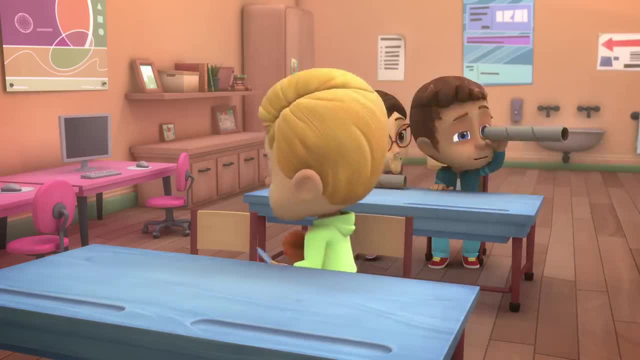 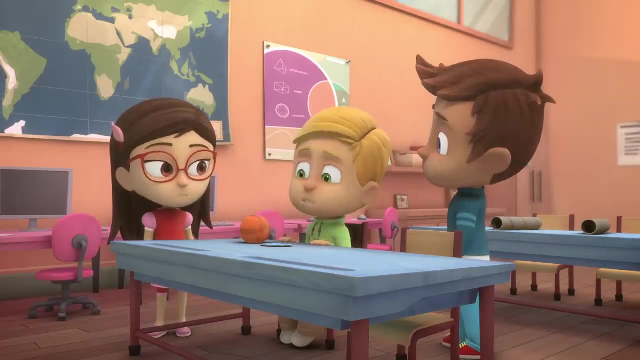 Aw, There's no more paper towel rolls. How am I supposed to make a rocket now? Maybe you can use something else. Amaya, there's only one way to make a rocket: With a paper towel roll. Come on, Greg. 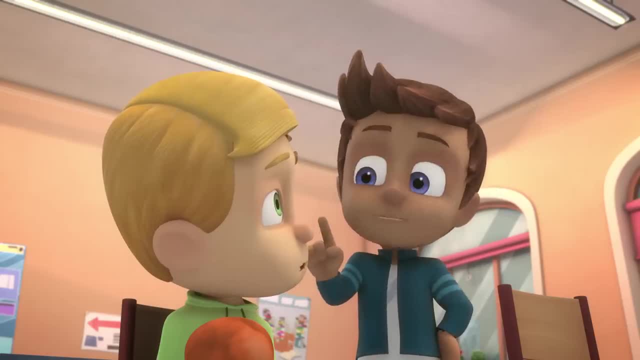 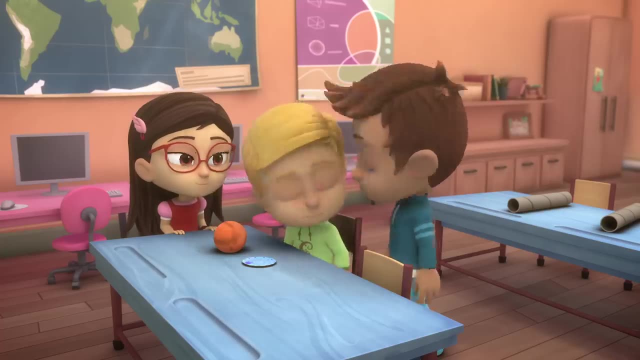 There can't just be one way to do anything. Maybe you'll be inspired after our trip to the Science Museum. There's even a rocket display- Really Awesome. Actually, the trip to the museum's been canceled, Oh no, Why. 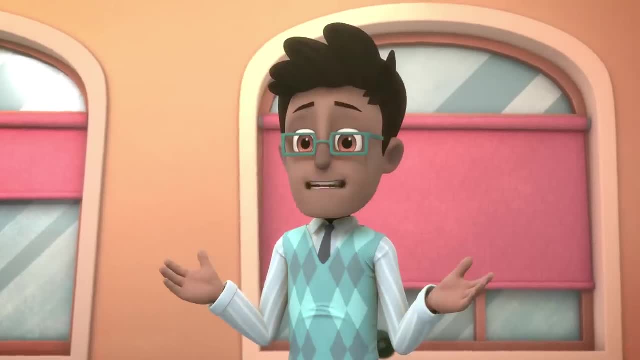 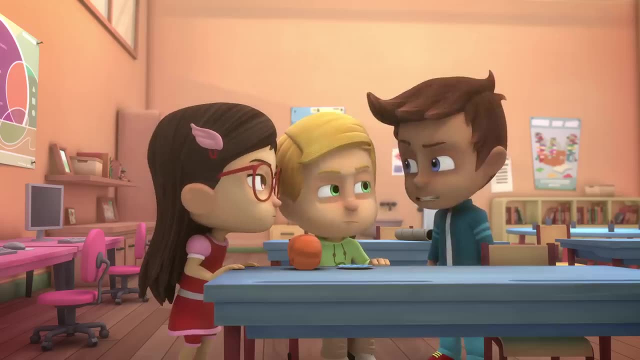 It's the strangest thing. All the buildings around it are fine, but the power is out at the museum. The lights are off and there's no electricity for the displays. That is strange And it's worth checking out to see if it's working. 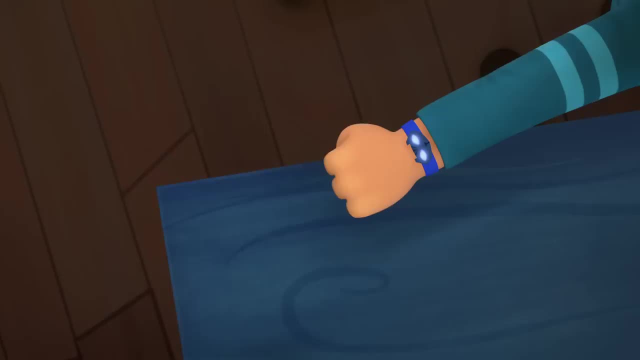 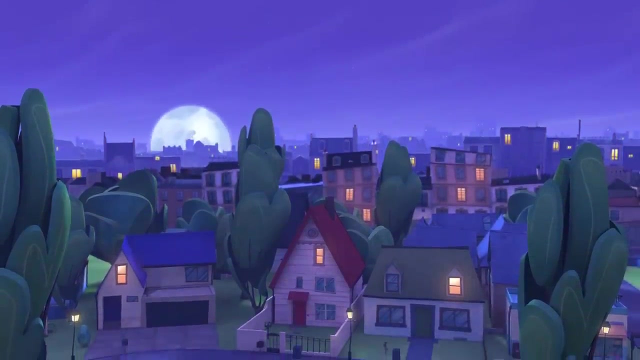 We'll be checking out tonight PJ Masks. we're on our way Into the night to save the day, Night in the city, and a brave band of heroes is ready to face fiendish villains to stop them messing with your day. 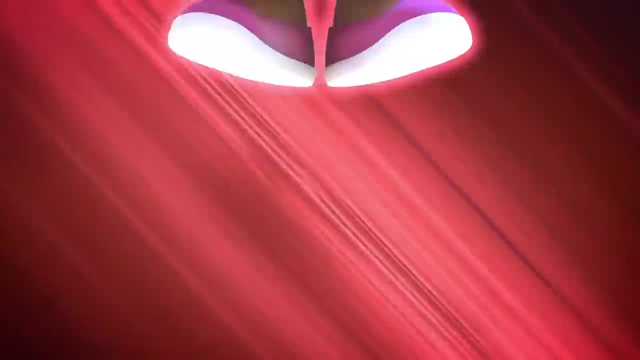 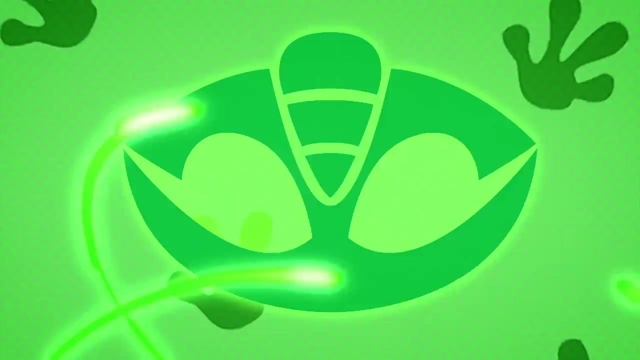 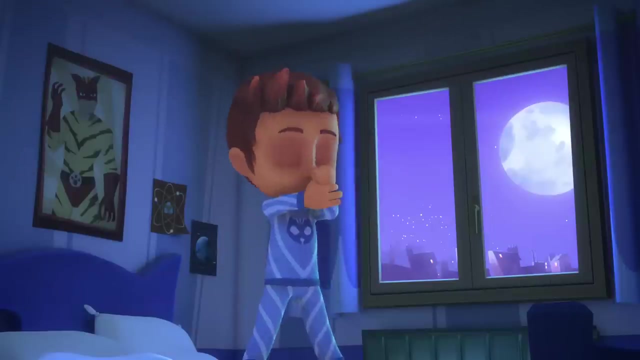 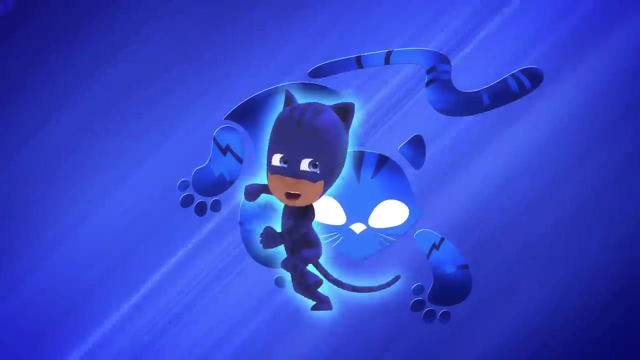 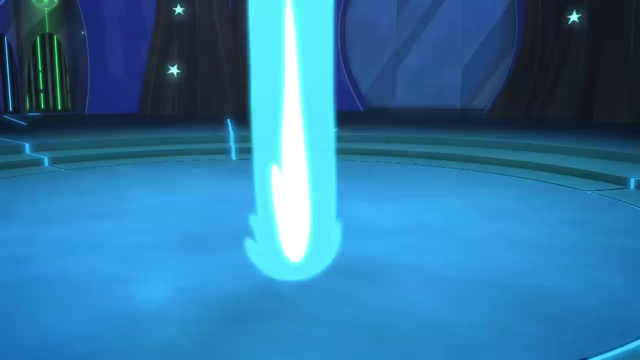 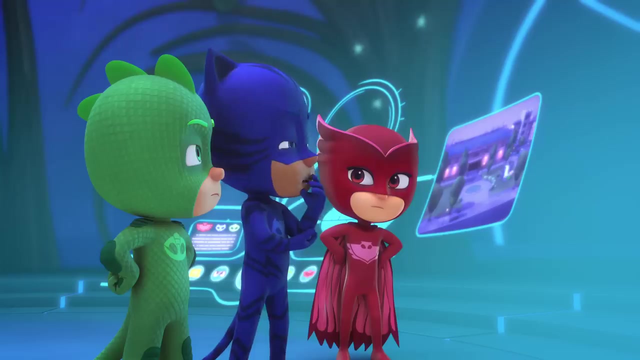 Ha-ha-ha. Amaya becomes Owlette. Yeah, Greg becomes Gekka. Yeah, Connor becomes Catboy. Ow The PJ Masks. That's weird. The lights are on at the museum. Didn't the teacher say the power was out? 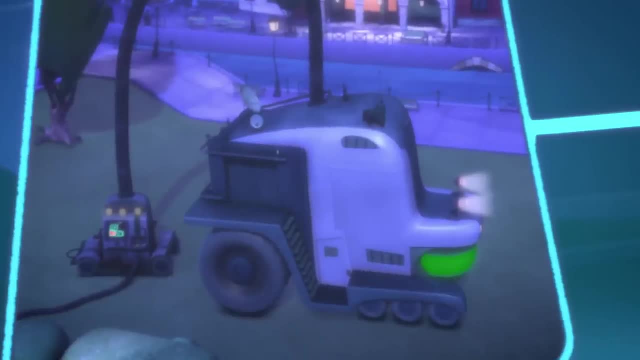 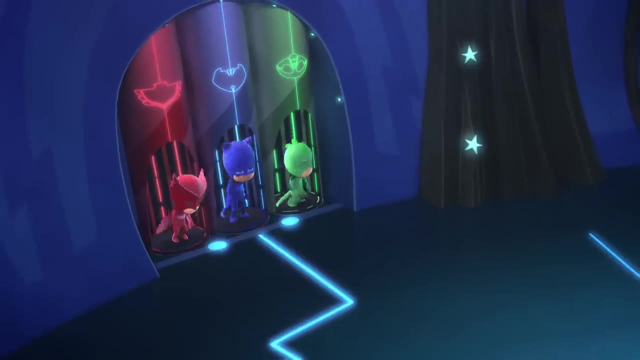 And that's not all. Look Gasping geckos, Romeo's lab. So that's who's behind this. To the geckomobile: Whoa, Wha, Whoa, Whoa, Whoa-o-o-o. 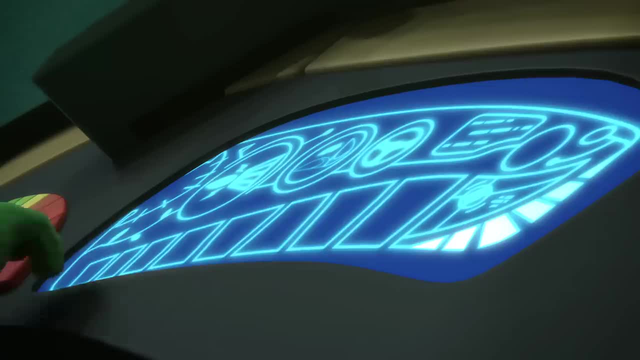 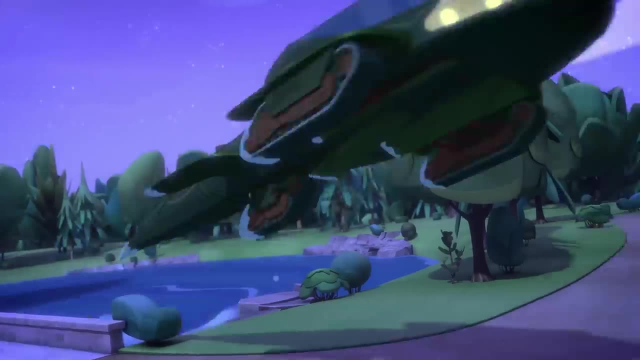 Whoa-o-o-o, Whoa-o-o-o, Whoa-o-o-o, Whoa-o-o-o, Ah, Whoa-o-o-o, Whoa-o-o-o, Whoa-o-o-o, Whoa-o-o-o, Ah, ah, ah, ah, ah. 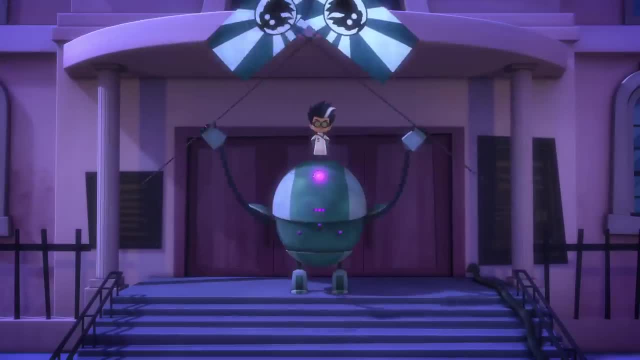 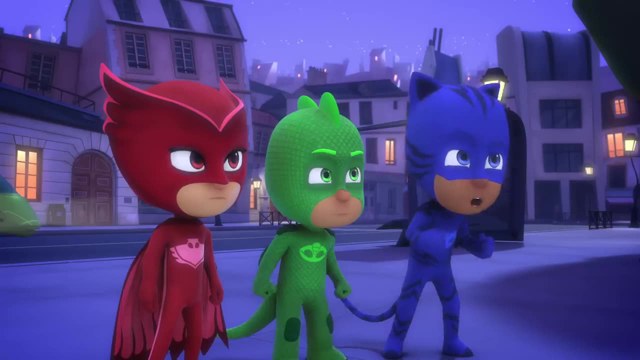 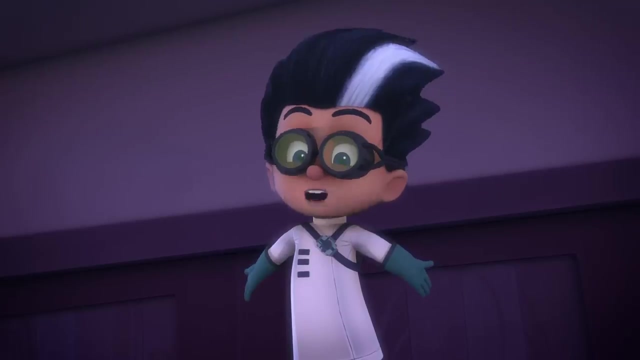 Yep, Definitely Romeo. How dare he take over the museum? That's right, I have taken over the museum. What are you up to, Romeo? My lab's battery needs to be charged and it's taking forever, So I've decided to use the museum as my base while I finish my big box of bad. 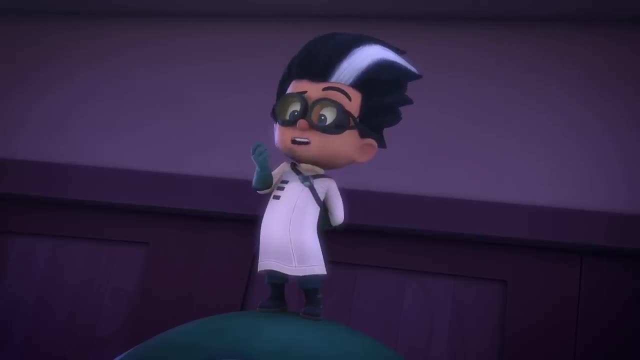 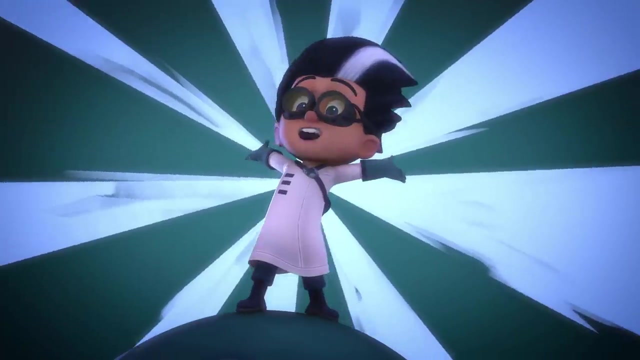 Big box of bad. Exactly When it's finished, it'll turn the whole city into my own private town dedicated to me. I'll call it Romeoville. I thought you were calling it Romeopolis. I haven't decided yet. 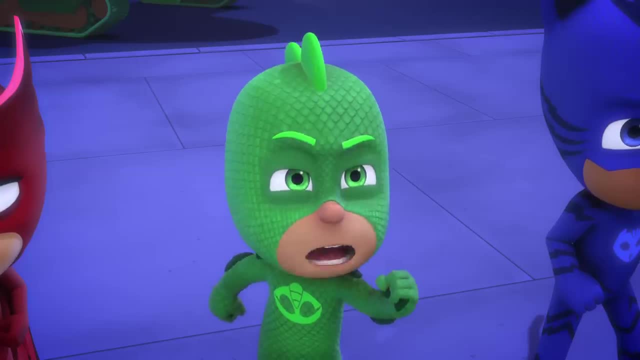 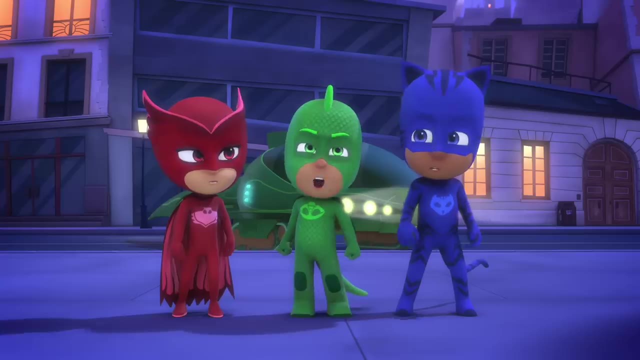 Forget it, Romeo. We're coming inside and putting an end to your plan. Oh, I don't think so. You see, I've booby-trapped the entire museum. There's no way you're getting in here. Oh, we'll see about that. 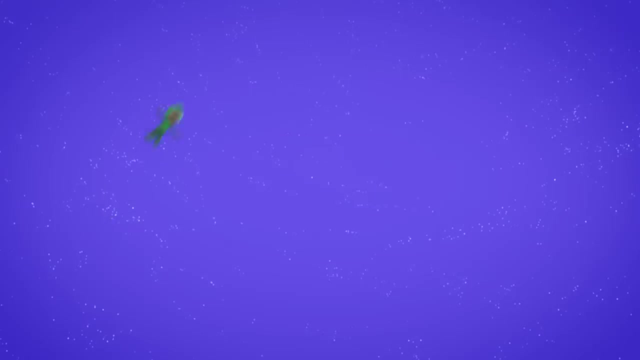 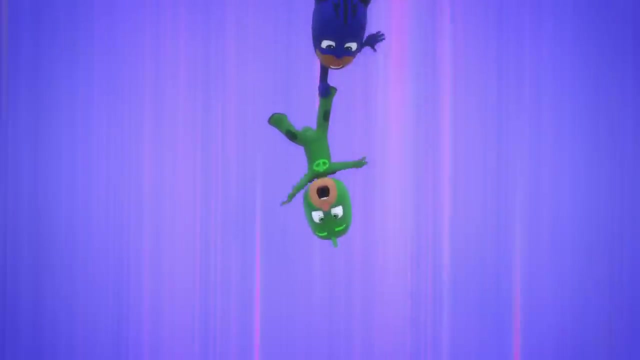 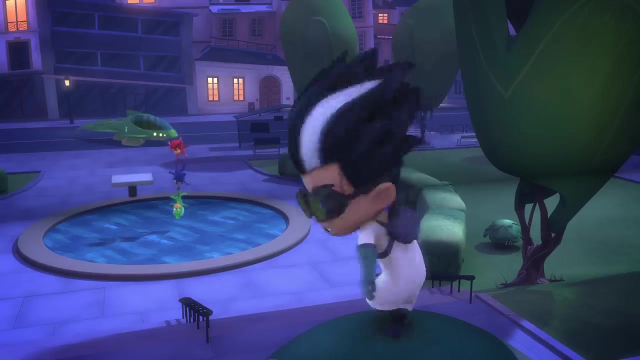 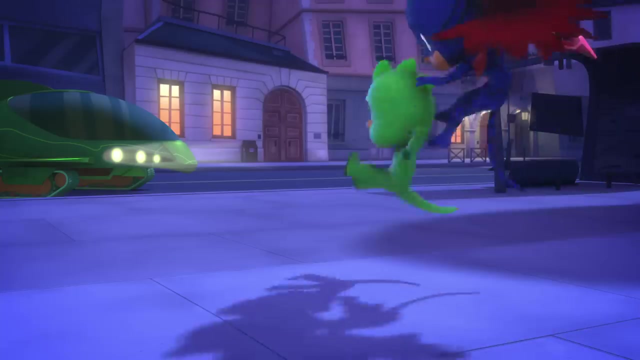 Gekko, stop, Uh-oh. Super Cat, jump Gotcha, Thanks. Thanks for testing out my booby-trapped lizard legs. Night-night PJ Monkeys, You okay, Gekko, I'm fine, But I'll be even better once we're inside. 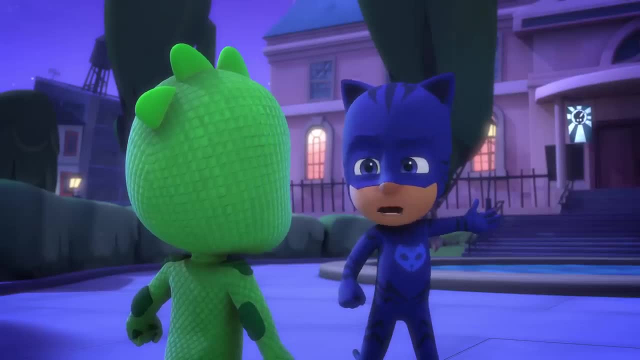 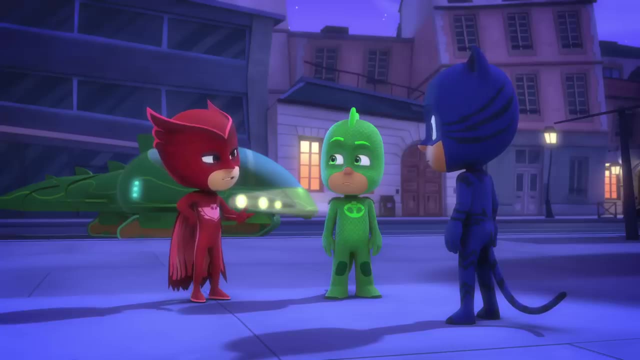 Gekko, you heard Romeo. The entire museum is booby-trapped. Maybe getting inside's not the answer, But getting inside is the only way to stop him. What if, instead of us trying to get inside, we try to get Romeo outside? 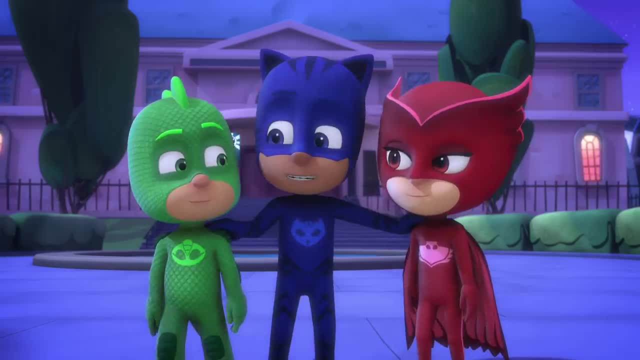 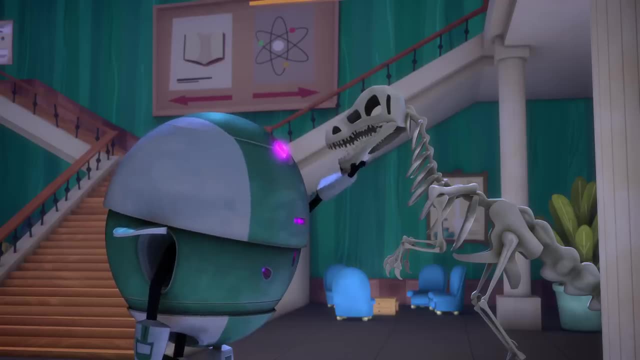 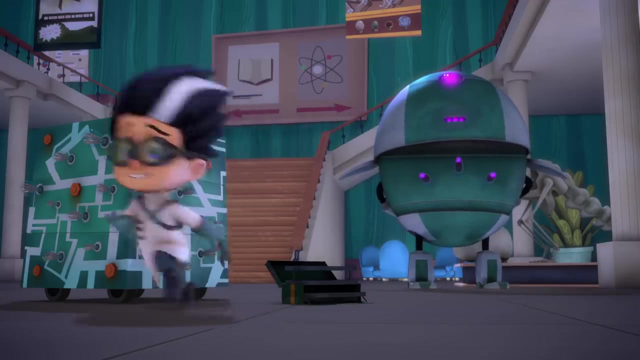 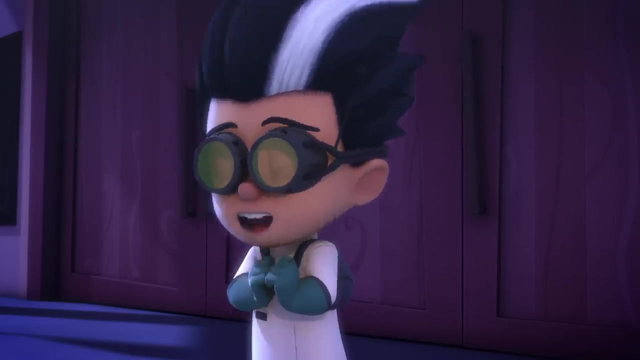 Great idea, Owlette, I think I know just the thing. Hello, I'm Robot, Hello Robot, My name is. Oh, I know that sound. It's an ice cream truck. I love ice cream. I hope they have double tofu pistachio. 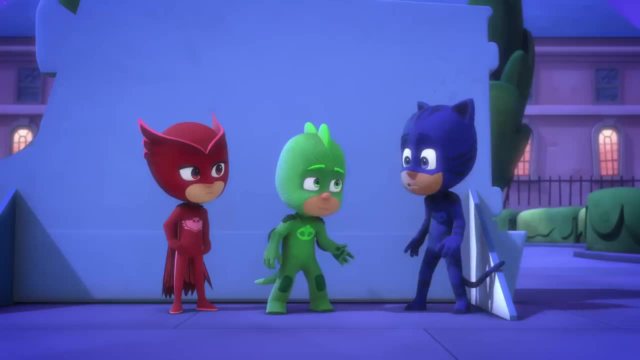 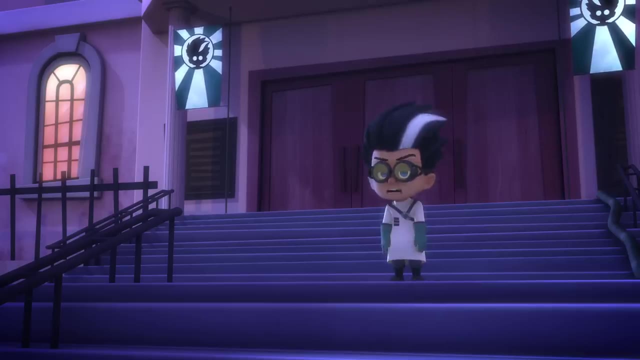 Woo-hoo, Romeo's coming, Now's our chance. Gekko, I've got you. now, Romeo, A trick. Ooh, I really wanted ice cream. Well, you'll pay for this. PJ Masks- Super Lizard Grin. 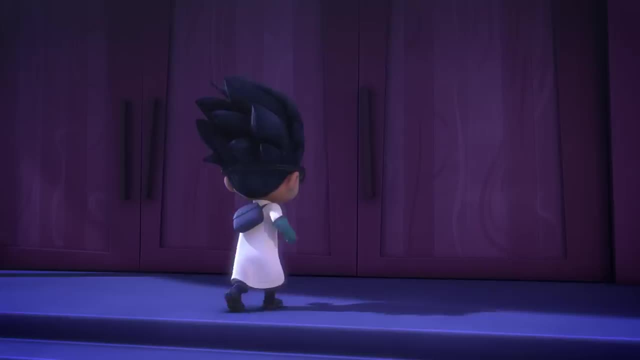 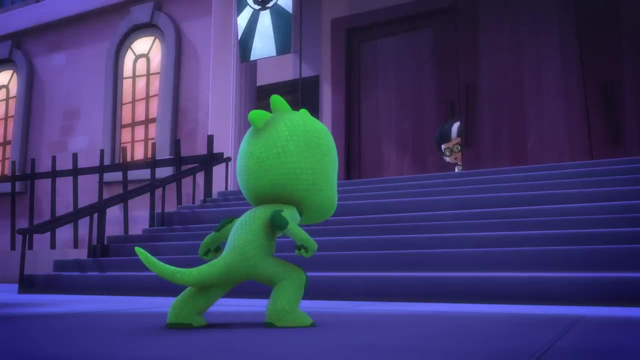 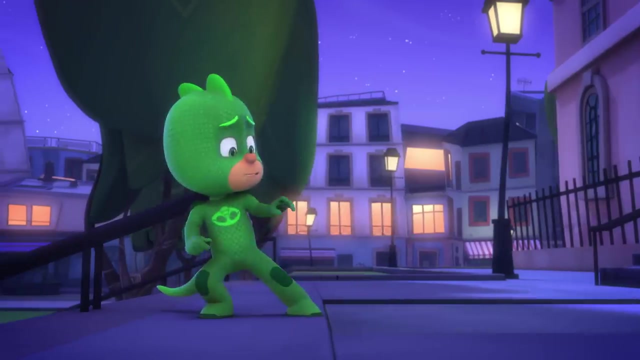 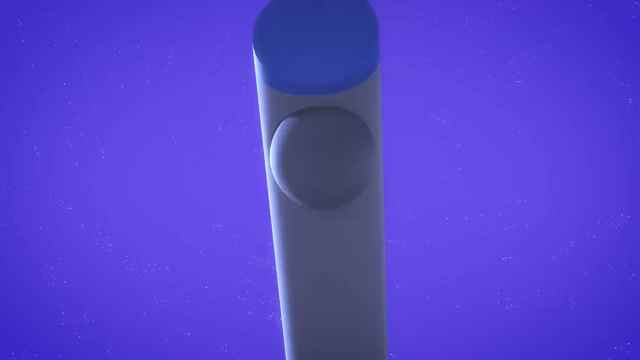 Gekko. You PJs never learn. Get back here, Romeo. What Ha You fell for it Again, Huh, Ah, Phew. Gekko, look out Gasping, Gekko, Phew. 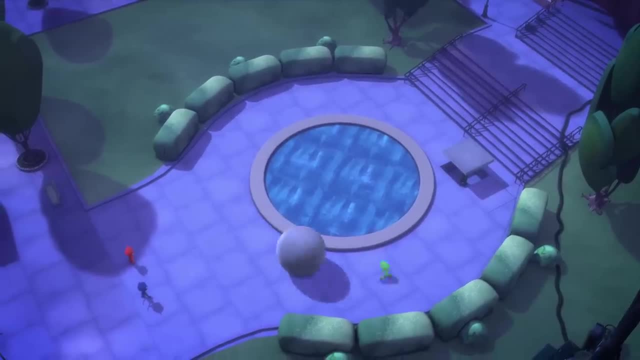 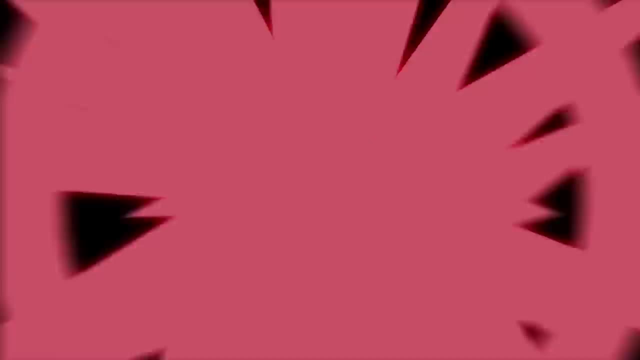 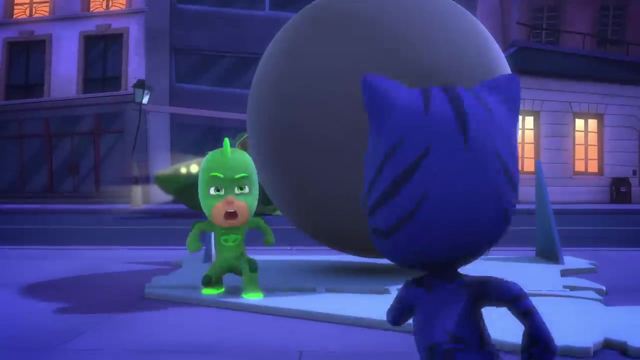 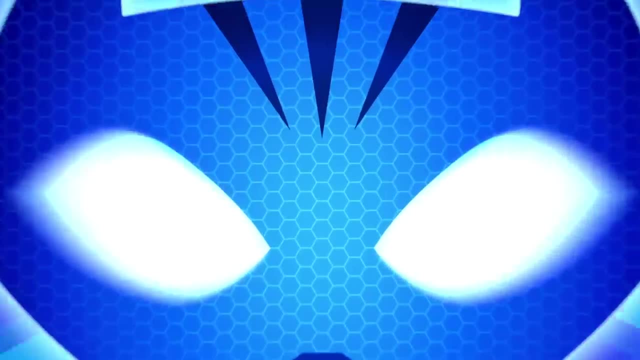 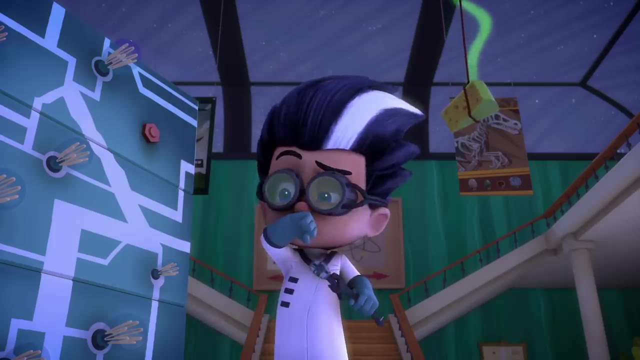 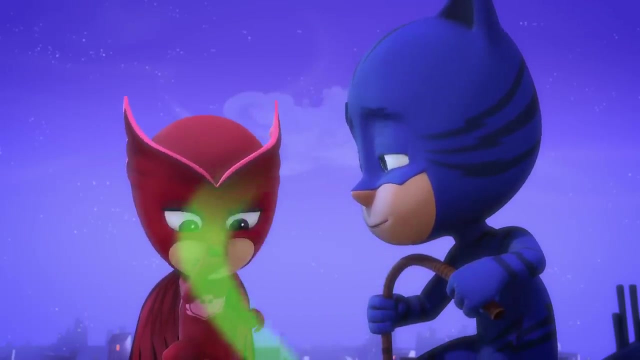 Hang on, I have another idea we can try. Oh, what is that horrible smell? This stinky cheese is sure to stink Romeo out of the museum. I sure hope so. I can barely stand to be this close to it. I can't take it. I need fresh air. 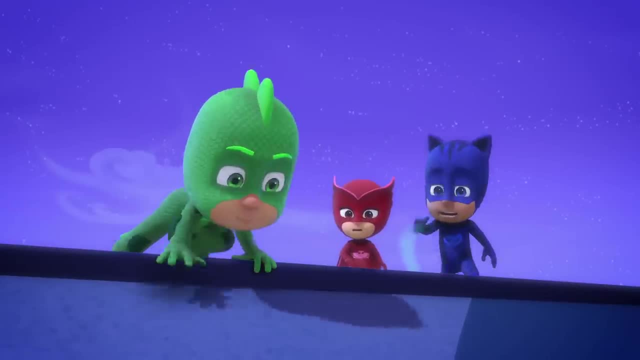 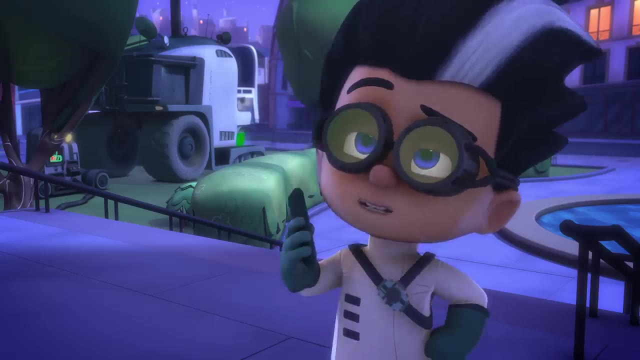 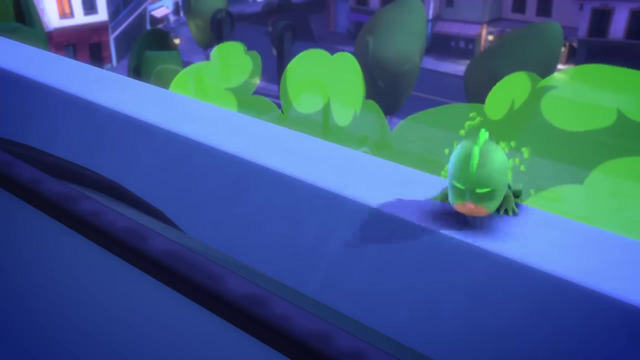 Romeo's outside, Gekko. hold on, I've got you now, Romeo, What I don't think. so Tonight's forecast calls for Stinky. Oh, super-duper smelly spray, Gekko, are you all right? 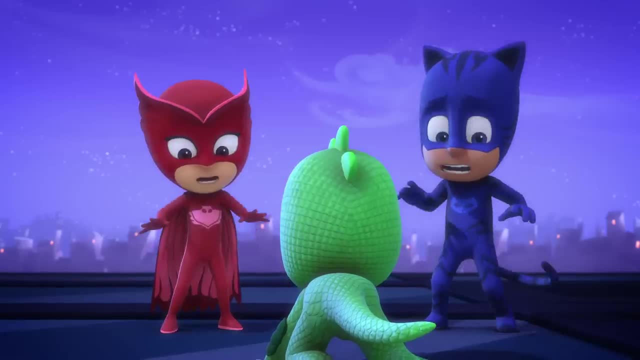 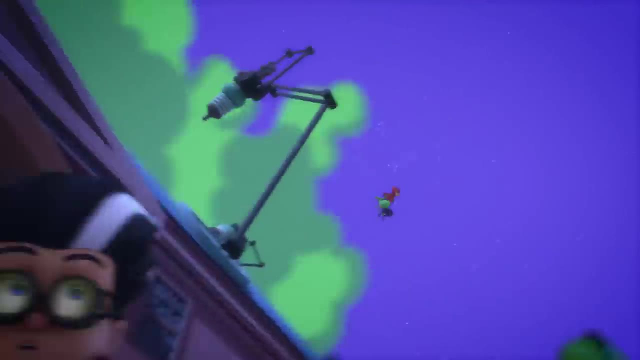 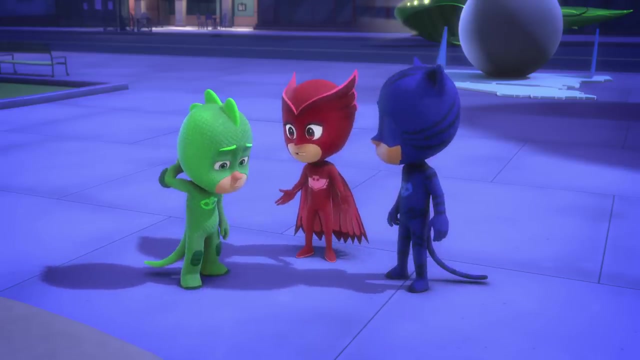 And now for the super-super stink Gekko. there's more than one way to solve a problem. Running after Romeo isn't working. Yeah, we have to keep Romeo out of the museum so that we can get in and get the big box of bad. 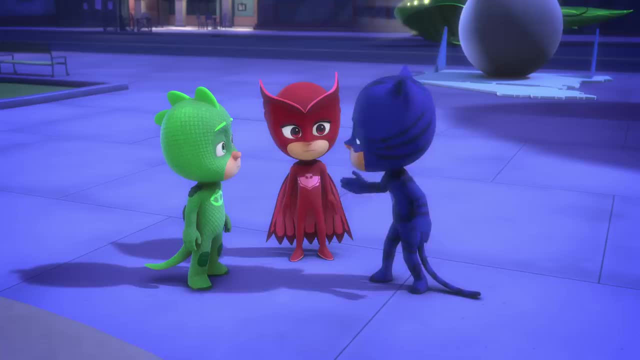 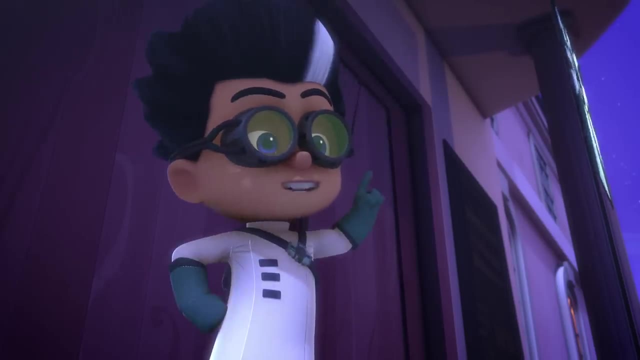 before it's finished. Too little, too late. PJ Stinks: I've finally finished my big box of bad. Ta-da, Uh-oh. I'm going to have to get my big box of bad. I'm going to have to get my big box of bad. 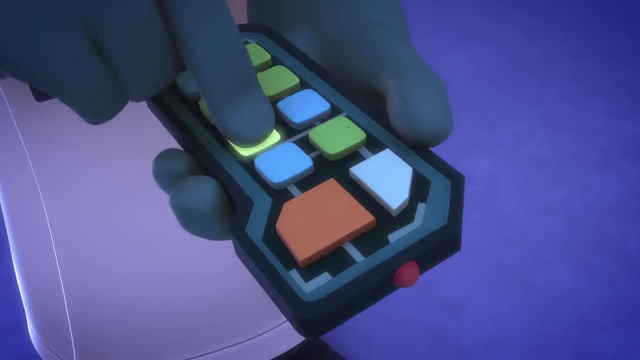 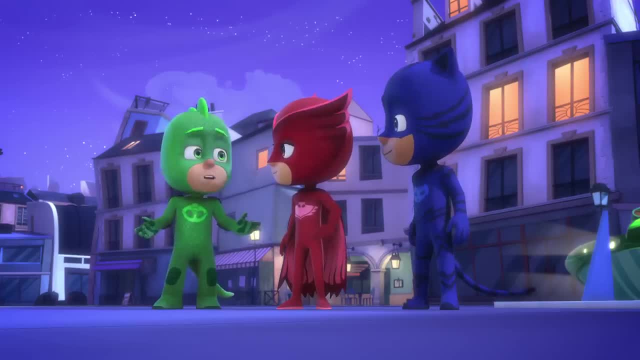 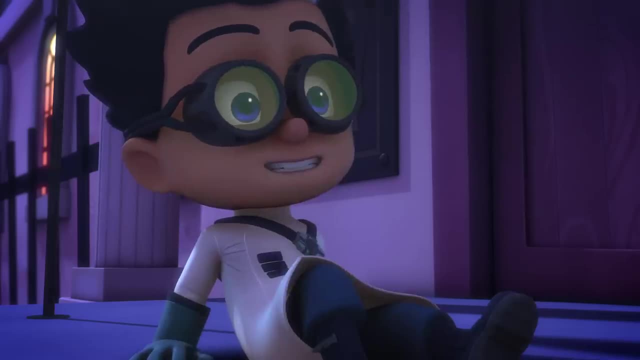 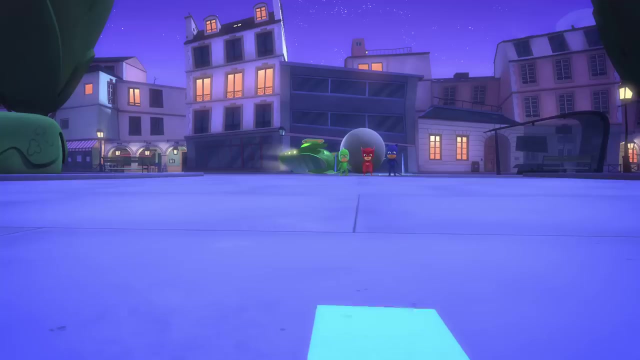 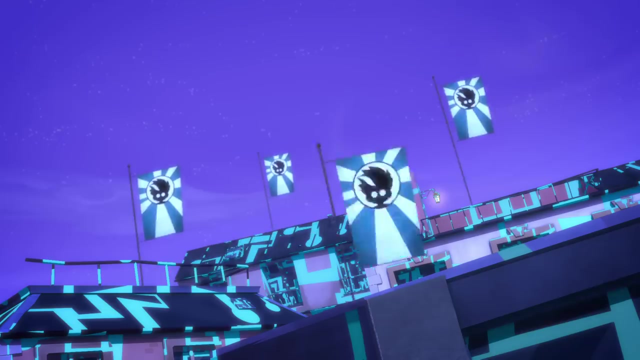 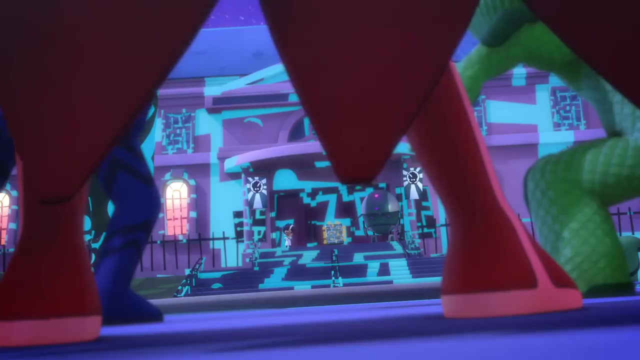 All that for a little flag. Well, I guess that's not so bad. Urgh, Skip the best part. Yes, Oh, look What's happening to the city, Don't you mean in Romeopolis? How are you doing this? 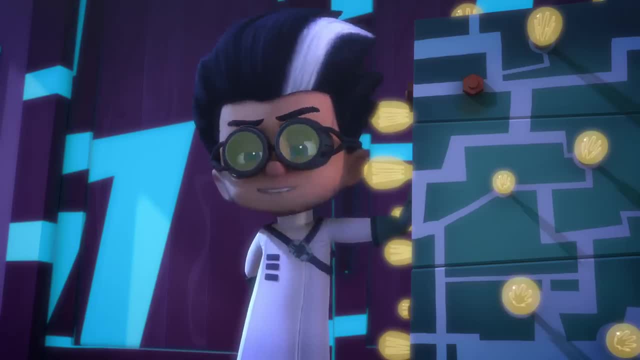 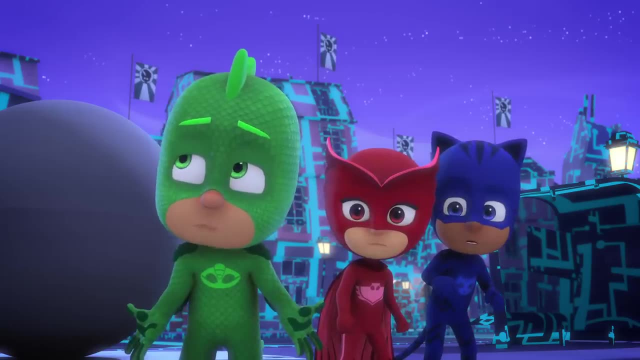 I'm not doing anything. It's all thanks to my big box of bad And some simple transfigure-modification. Oh, this is all my fault. I kept trying the same thing over and over again to stop Romeo, If I hadn't been so focused on doing things right. 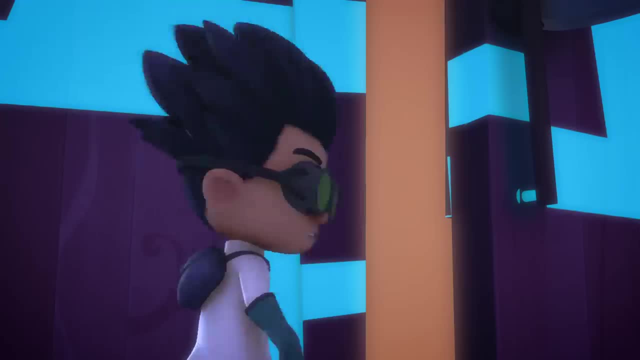 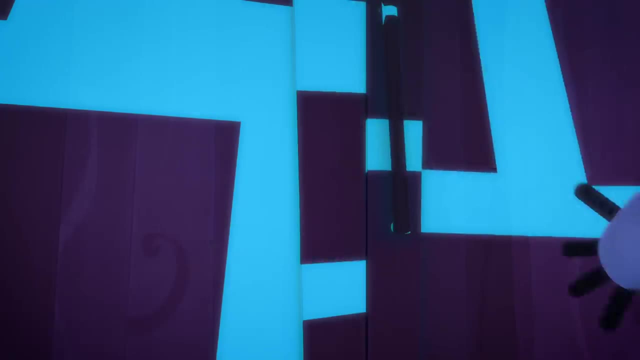 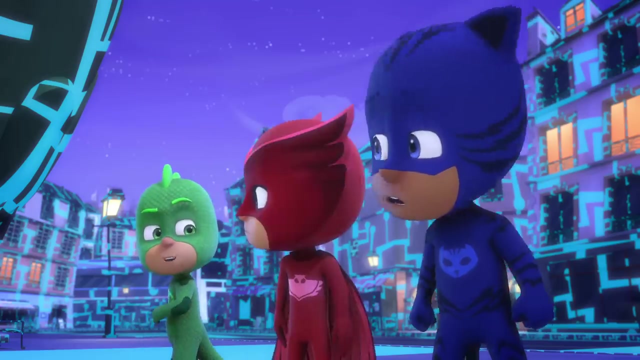 Romeo would have never finished his big box. That's big box of bad. If you're looking for me, I'll be inside On my swoon. We're never getting in there. Huh, You're right, Catboy, But maybe there's a way to get Romeo out here. 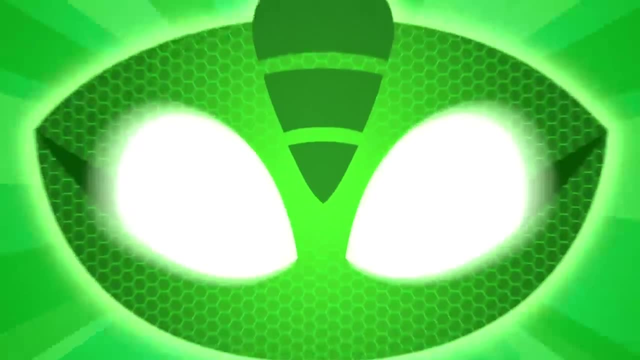 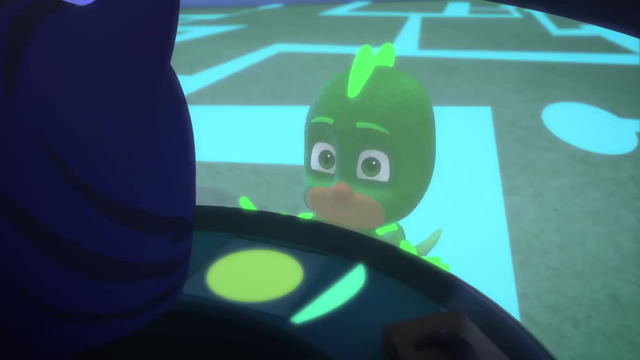 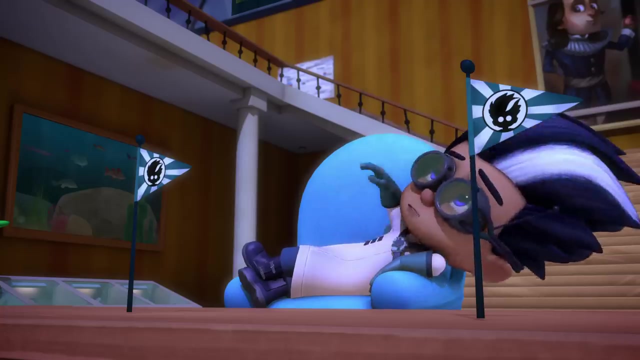 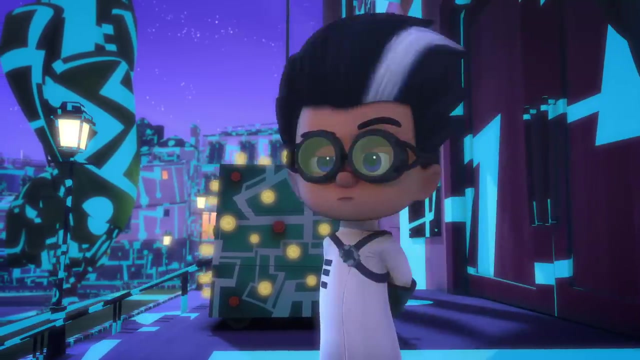 It's time to be a hero. Uh-oh, Now do I want to be Mayor Romeo or King Romeo? Master, you need to look outside What My lab is moving. That's impossible. It's not charged. Ah. 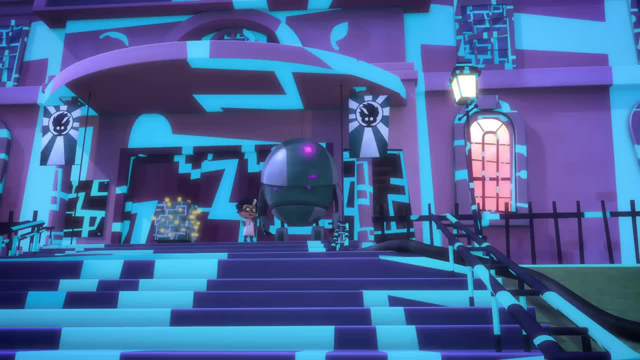 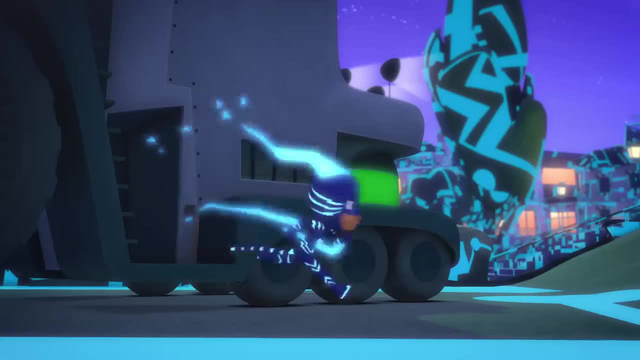 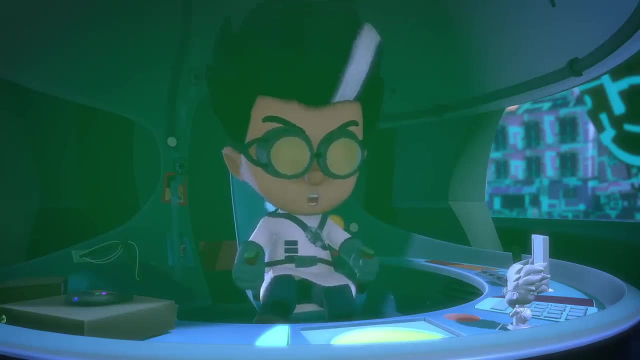 Get out, Get out Robots. Super Catboy, I'm going to get you, I'm going to get you. Ah, And feed What? Where would it go? It was just moving. Yeah, it was moving, Thanks to my super gecko strength. 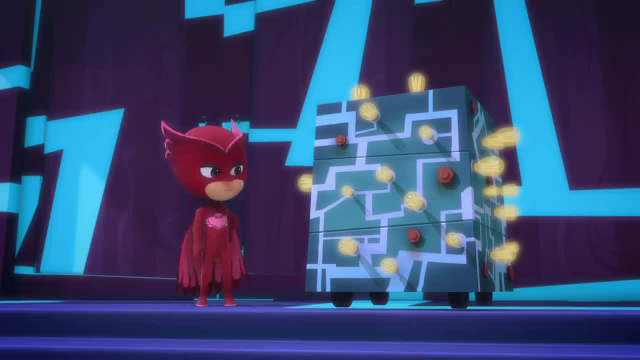 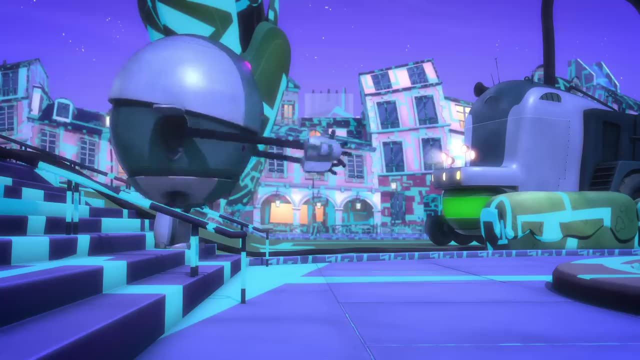 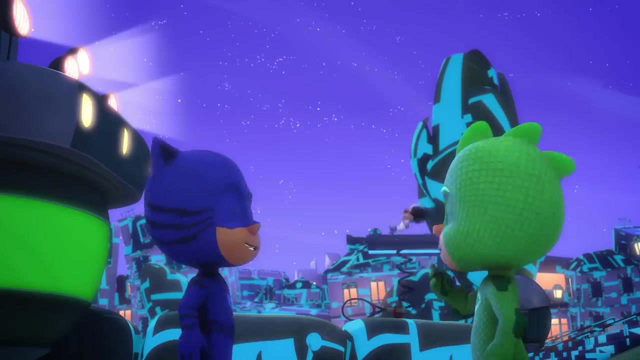 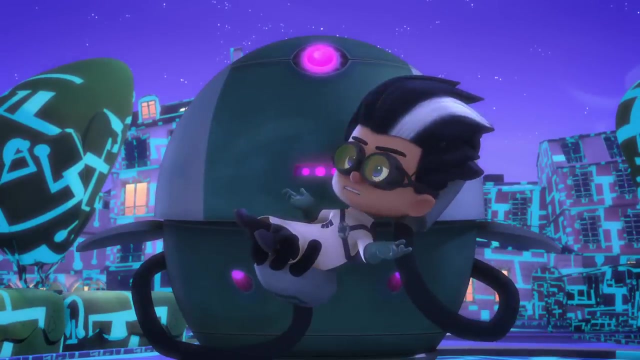 You tricked me. My box, No, Master, remember the Booby traps? Ah, Ah, Whoa, Whoa, Are you all right? I'm fine, As long as we don't step on another Booby trap. 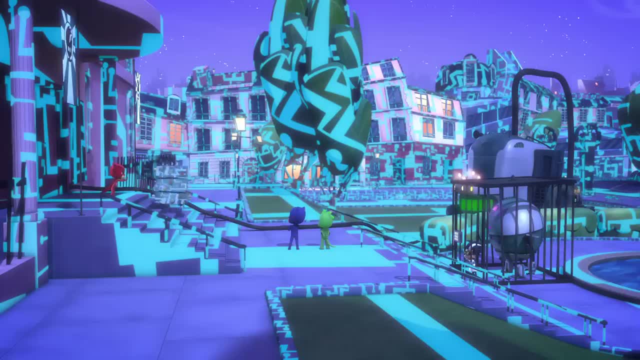 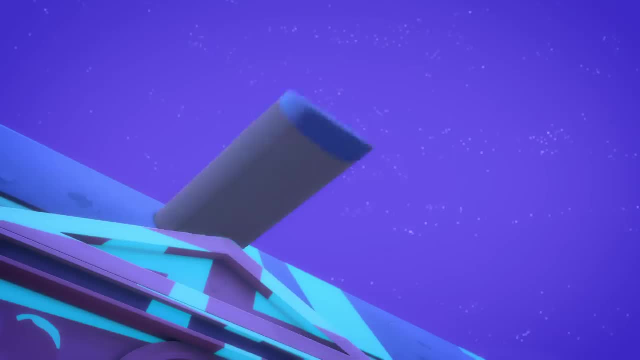 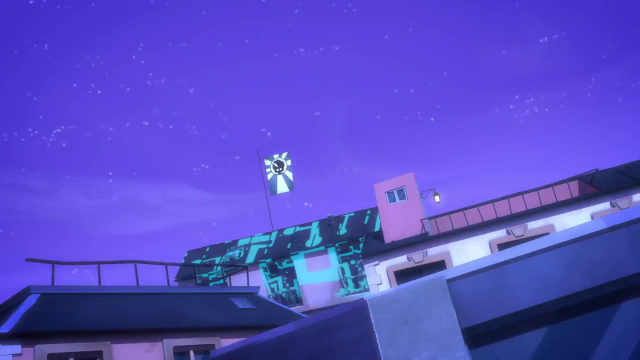 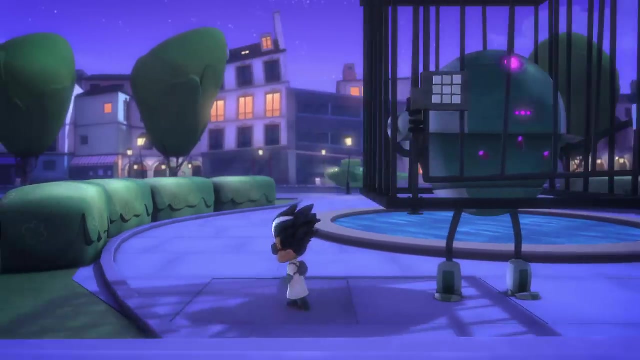 My big box of bed. Whew, It's okay, Is it It? DOTS, ninnyso flipped it over. Yeah w chưa Francisco, you failed. No, Lysolikas, Noooooooo, Lysolikas pomer. 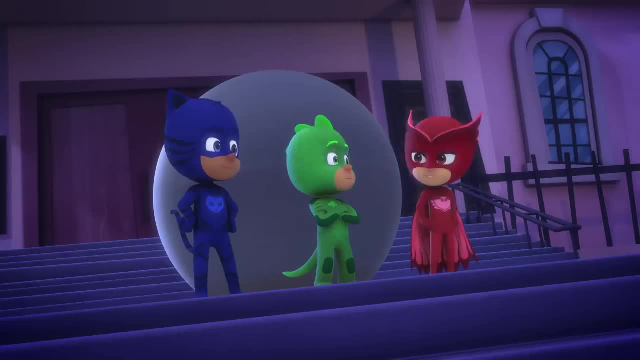 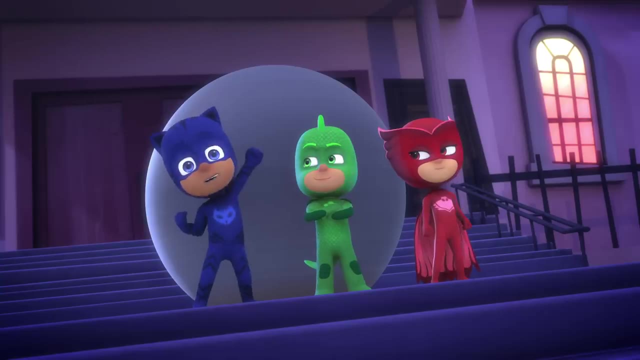 promise is still here. What am I doing? P-Joland Agh, Get him out, Get him out. I don't want to deal with him anymore. No, All shout hooray, because in the night we save the day. 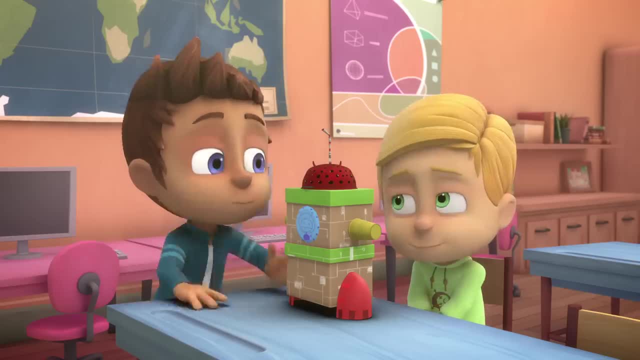 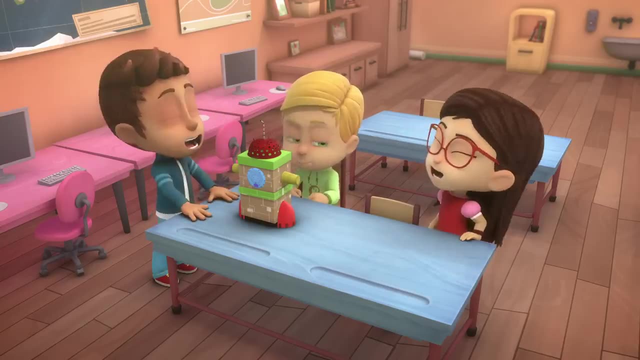 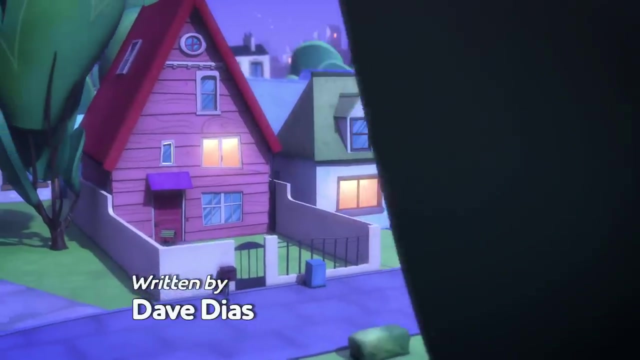 Like it, I love it. It sure is unique. I was inspired by seeing Romeo's box last night. I call mine the big rocket of amazing Owlette and the Battling Headquarters. Greg Connor, do you read me Over? 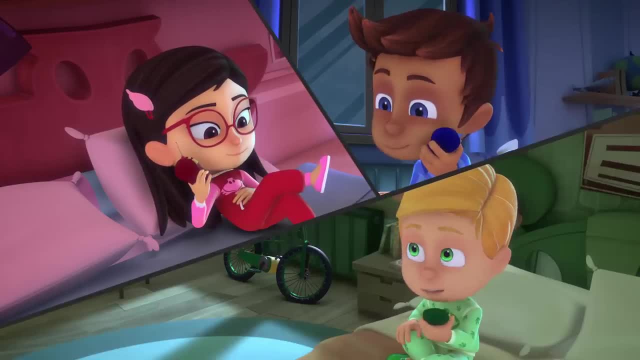 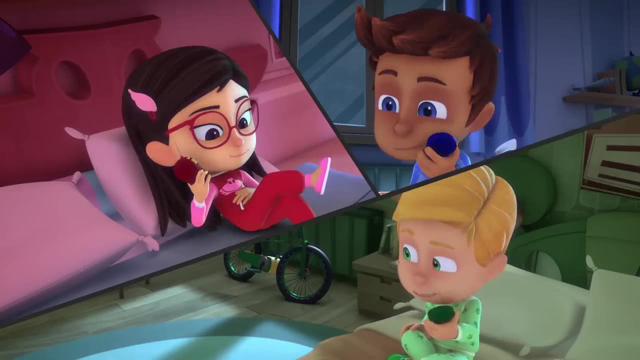 We hear you loud and clear. Amaya, Me too Over. You guys wanna go bike riding tomorrow morning? Sure, that sounds like fun. It'll be extra fun for me. I just got a new bike for my birthday yesterday, Cool. 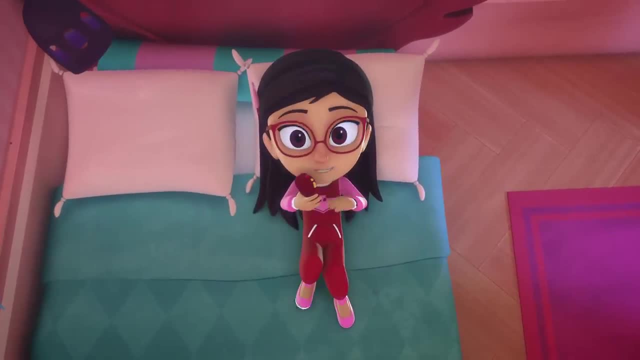 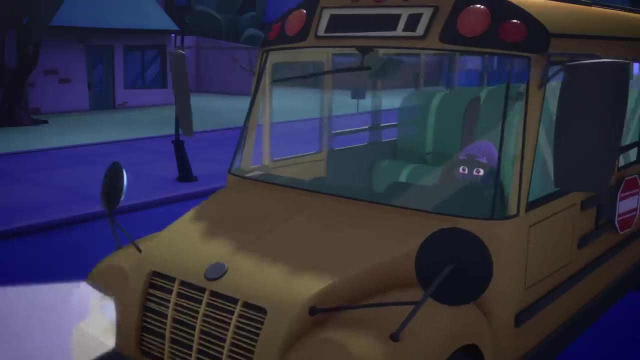 A new bike. I totally want a new bike too. Huh, What was that? It's a school bus And there's a Ninjalino driving it And there are more buses right behind it. I love it, I love it. 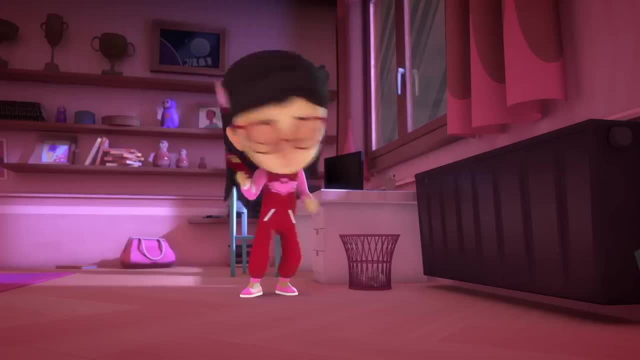 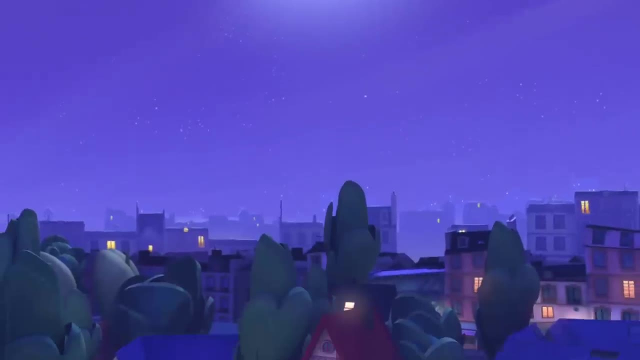 I see him, I see them. We need to find out what's going on. PJ Masks. we're on our way Into the night. we save the day Night in the city, and a brave band of heroes is ready to face fiendish villains. 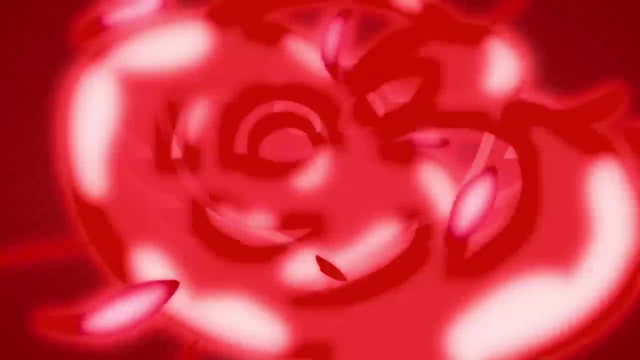 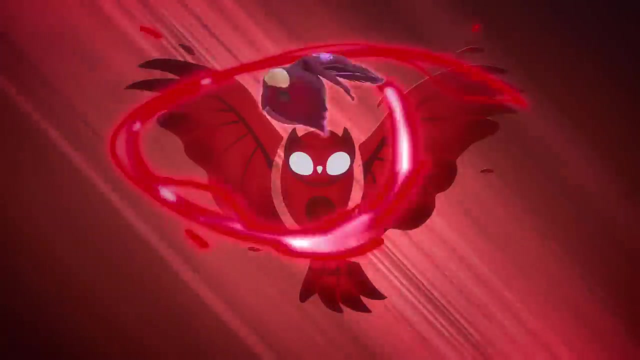 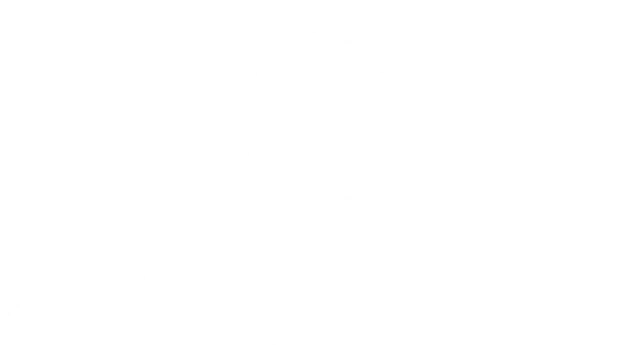 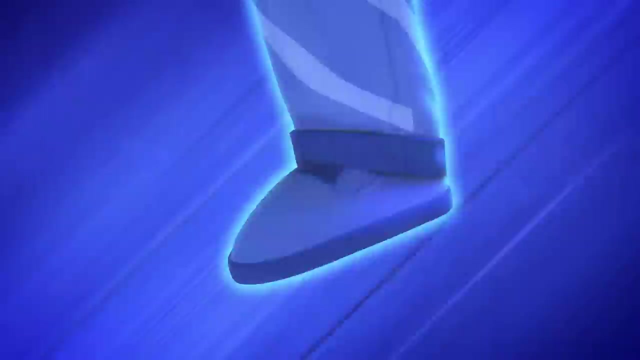 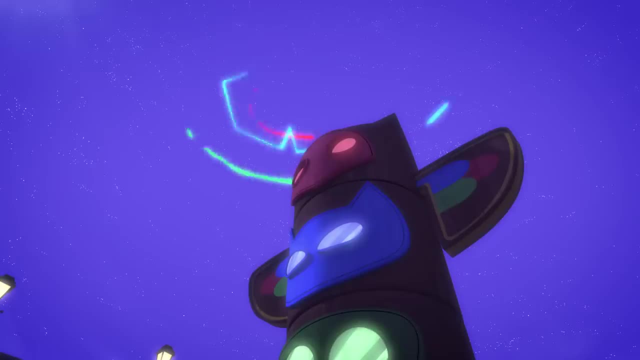 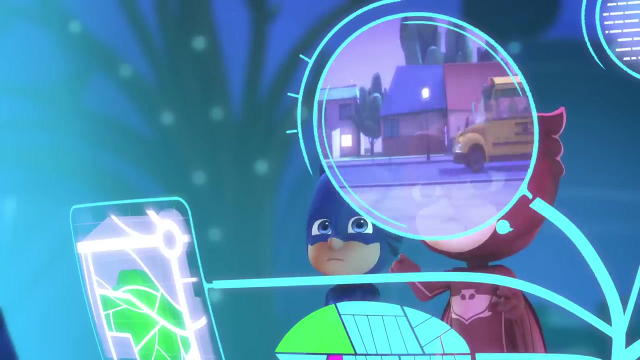 Catboy, Catboy, Catboy, Catboy, Catboy. The PJ Masks, The PJ Masks. We need to find out where the Ninjalinos are taking those buses. Uh guys, I think I know where they are Look. 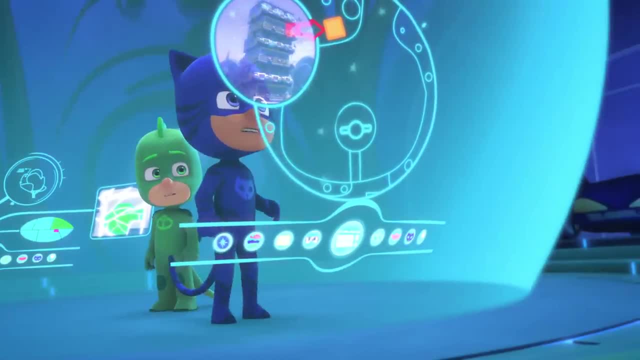 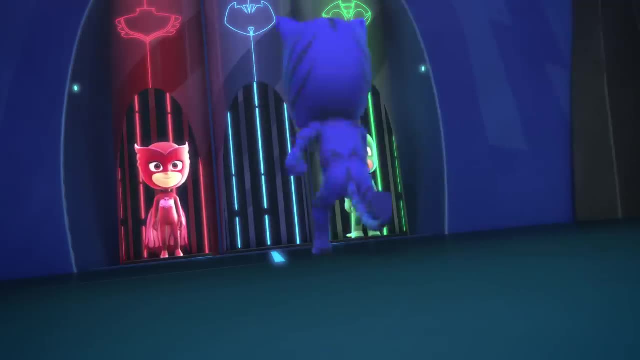 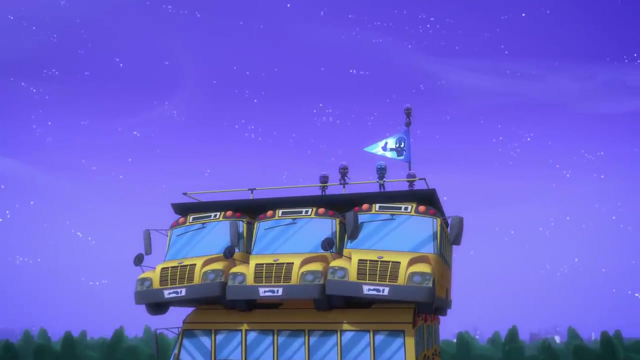 Night Ninja. The buses are in the park right next to our headquarters. What's he doing with them? There's only one way to find out: Come on, Look how tall his bus tower is. PJ Masks. Isn't it a lovely night to park in the park? 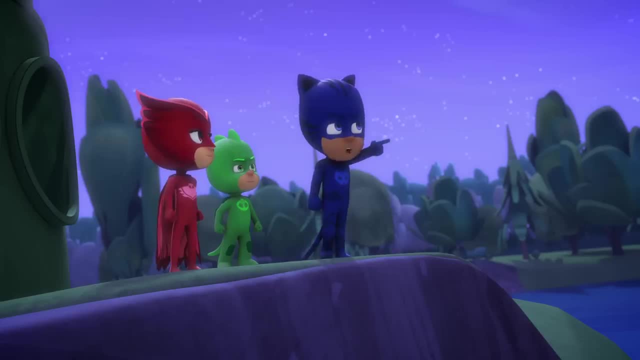 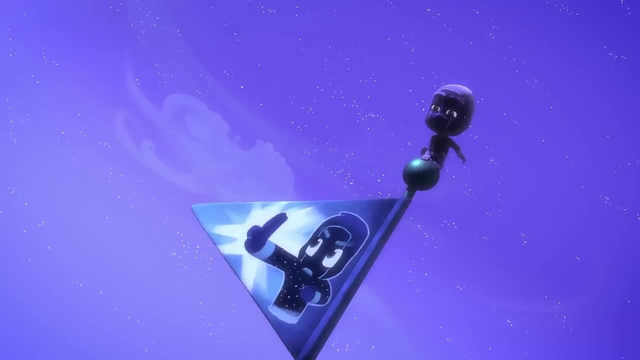 Night Ninja. What are you doing with all those school buses? Put them back in the bus? I don't think so. Say hello to my Fortress of Fury, the best headquarters ever. Sorry, but we already have the best headquarters ever. Now put those school buses back so kids can ride them to school. 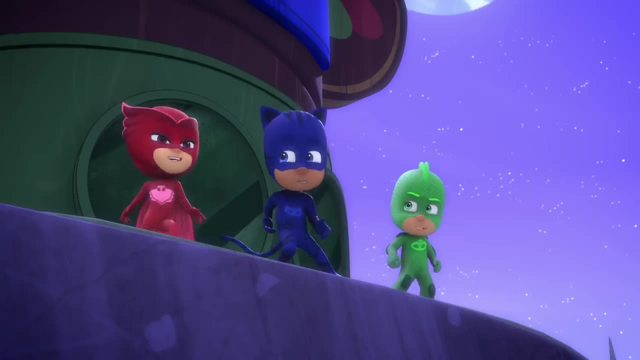 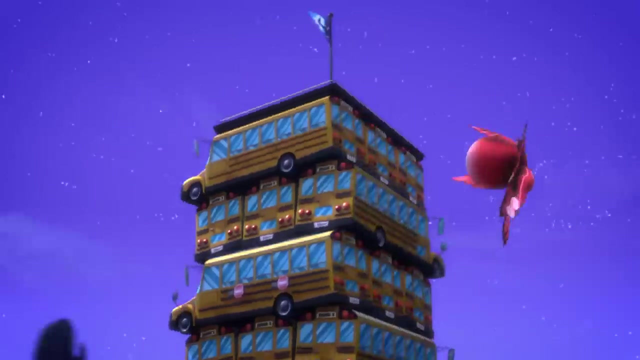 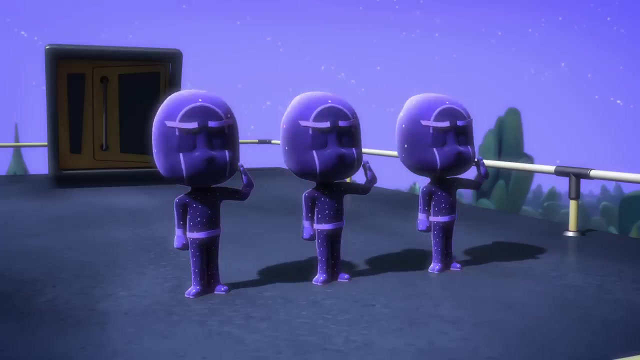 Make me. I'll fly up there and see if I can get a closer look. Super Owl Wing Ninjalino, let's give the noisy bird girl a nice loud hug, Okay, And a nice warm greeting, Hi-yah. 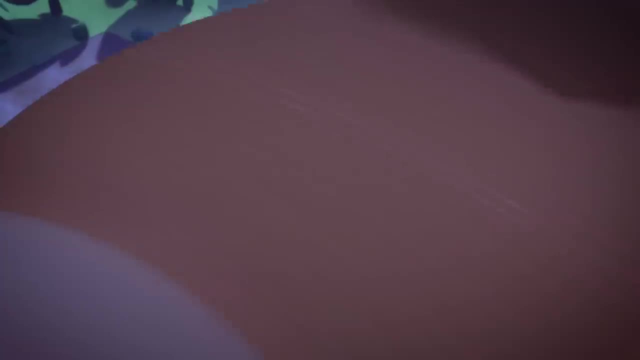 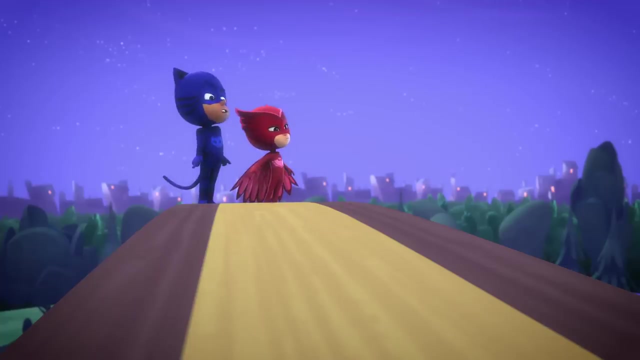 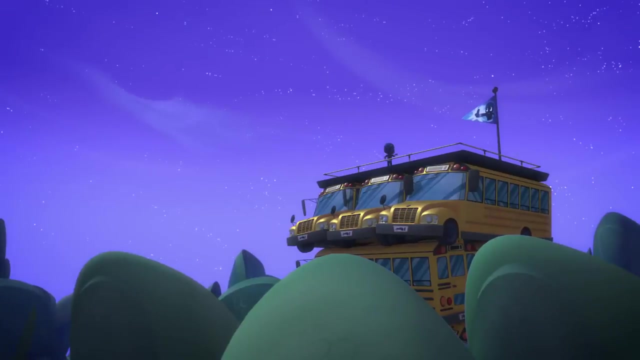 That's loud. All right, Super Gekko Muscle, Super Cat's Feet- Phew. Thanks, Catboy. That's it Night Ninja. We're taking you down. I'm sorry, Did you say something? My fortress is so loud I couldn't hear you. 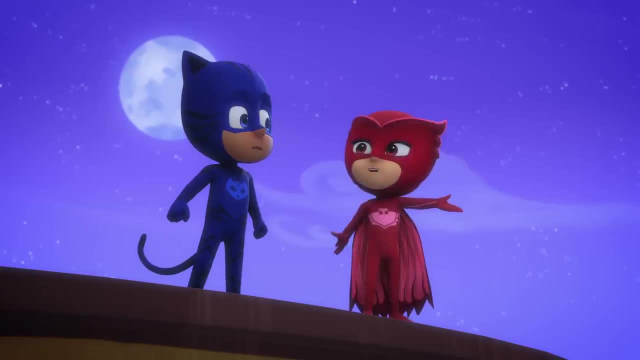 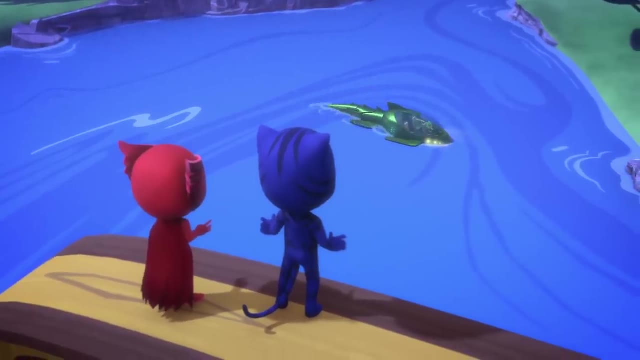 That horn defense is pretty powerful. We should totally get it for our headquarters. Why We don't need noise? Our base has lots of stuff to stop Night Ninja Guys. let's use our vehicles to stop his fortress. We could, Or we could, use a new noisemaker to stop him. 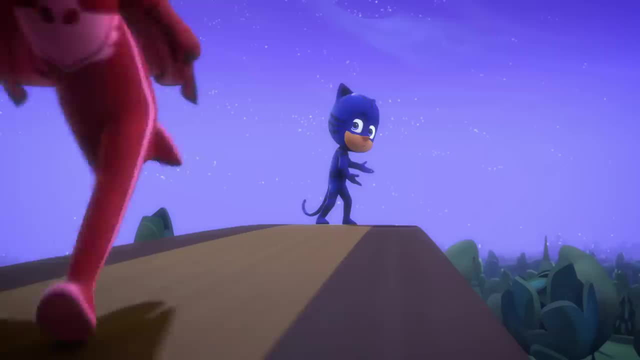 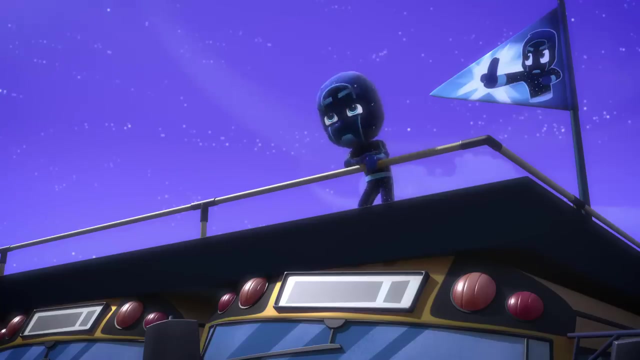 But Owlette, just because he has one doesn't mean you need one too. To the Cat Guard: What are you, PJ Pests, going to tell me how great my fortress is? Go on, say it. Never We're taking those buses back. 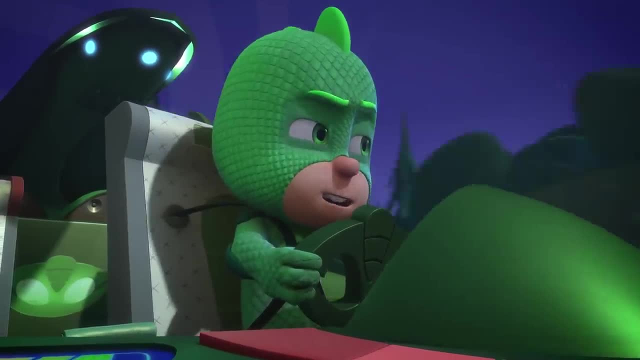 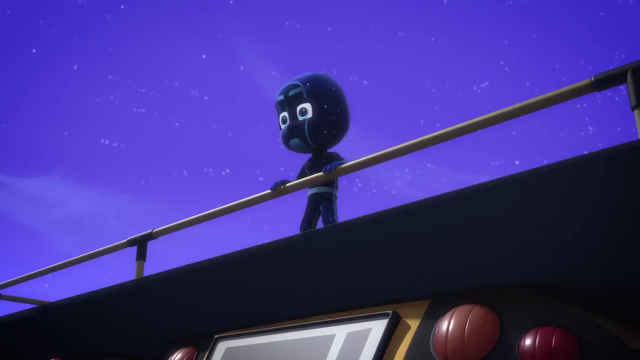 Catboy, I'm going to knock all the buses loose by whacking them with my tail. Great idea, Gekko, And I'll make sure they don't get damaged. Uh-oh, It's starting to rain- sticky splats. 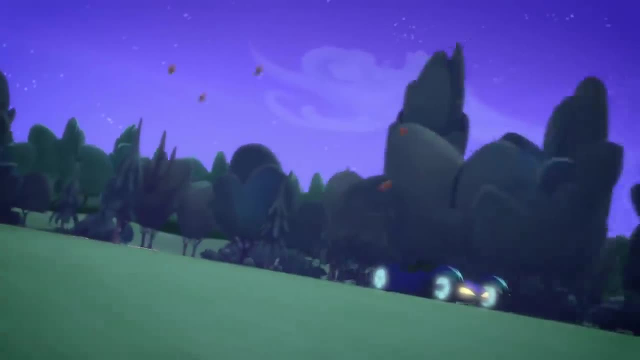 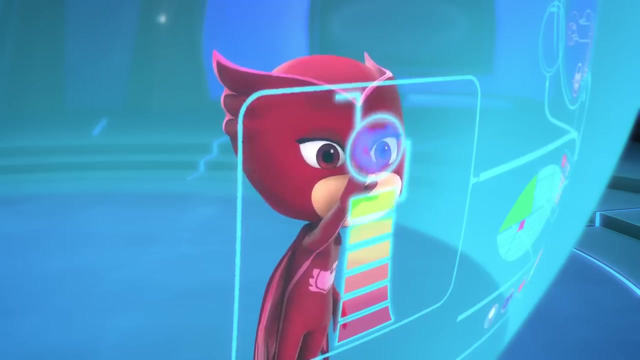 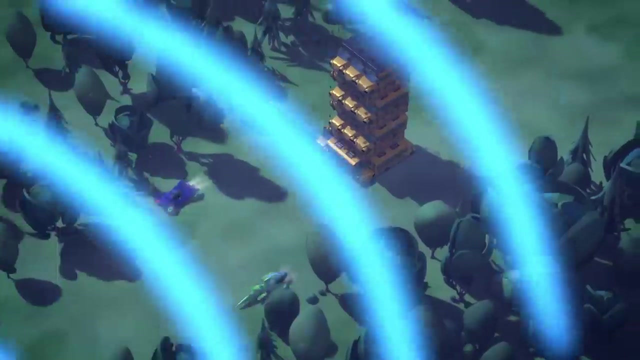 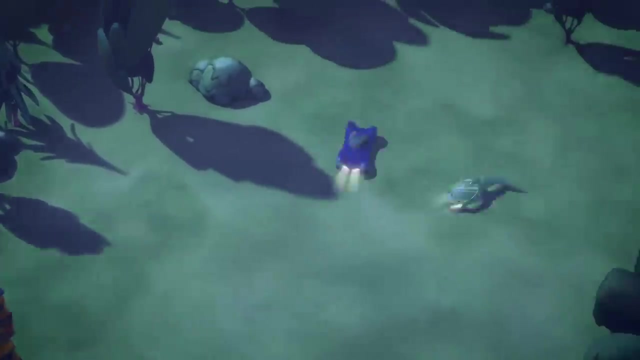 Sticky splats, Sticky splats There. Listen to this noise. Night Ninja. It's the cat's meow, Here comes the tail. Whoa, Whoa, Ha, Ha-ha. My fortress is built, ninja, tough Ah. 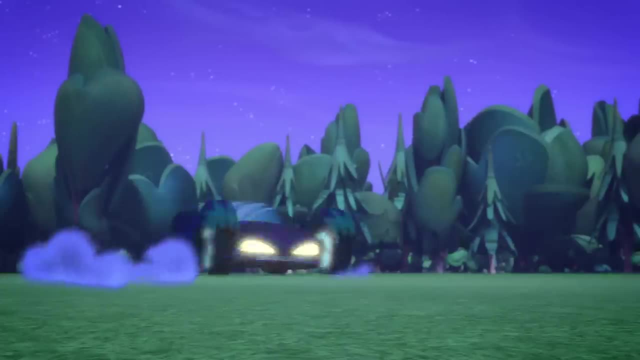 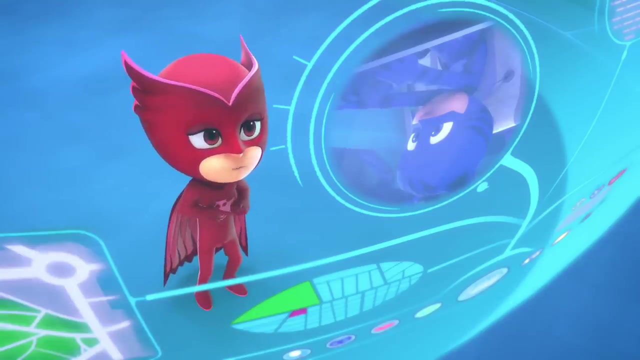 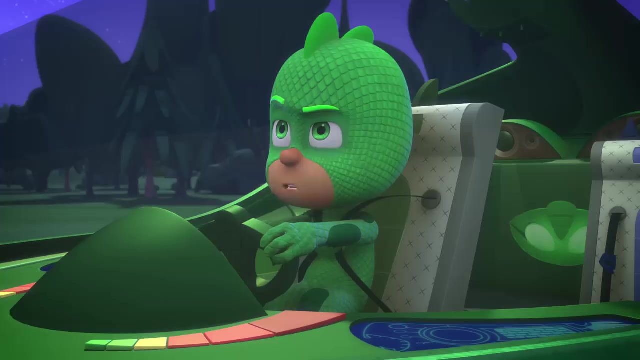 Ah, You'll have to do better than that to knock it down. Sorry, Catboy, I didn't know the mega-meow would make you spin out. Yeah, that mega-meow was more like a mega-mistake. Looks like it's up to me. 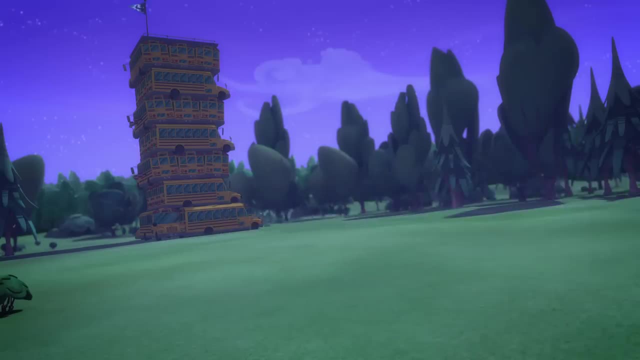 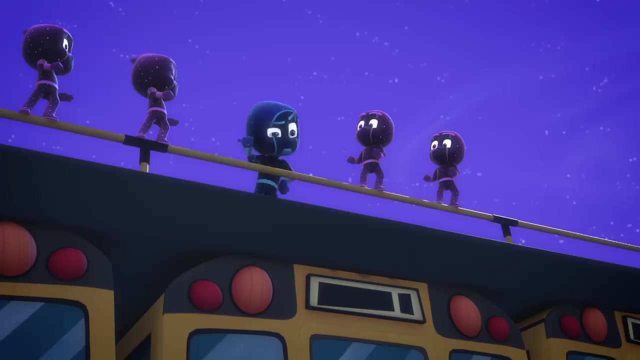 Gekko-mobile camouflage. Where has that goofy Gekko gone? Huh, Ninjalino, why are you out on the buses? Get back in the buses and stop Gekko. Ha, Ha, Ha, Ha-ha-ha. 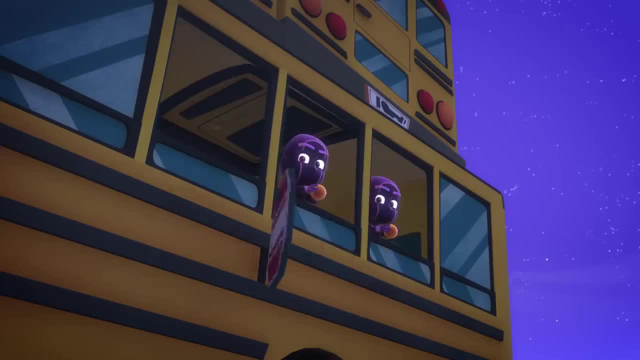 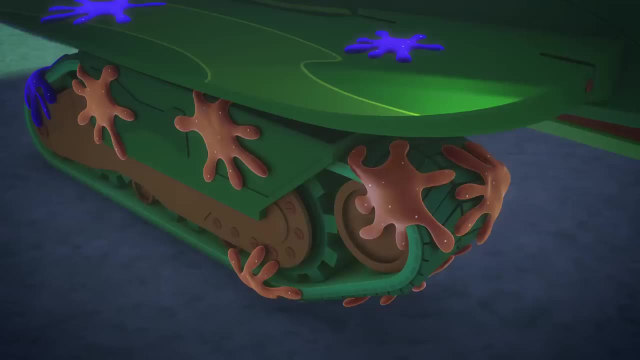 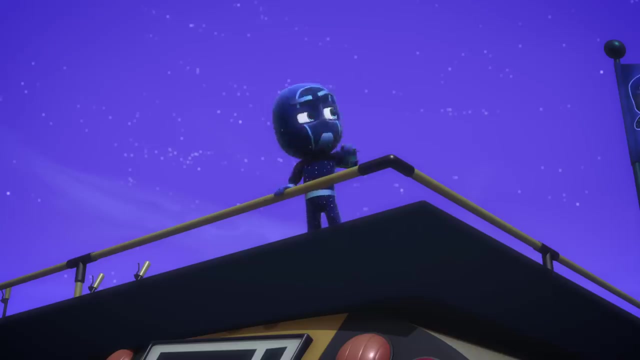 Ha-ha-ha, Ha-ha, Ha-ha, Ha-ha, Ha-ha, Gasping Gekkos, I'm stuck There. you are Ninjalinos, let him have it. Uh-oh, Looks like this is my stop. 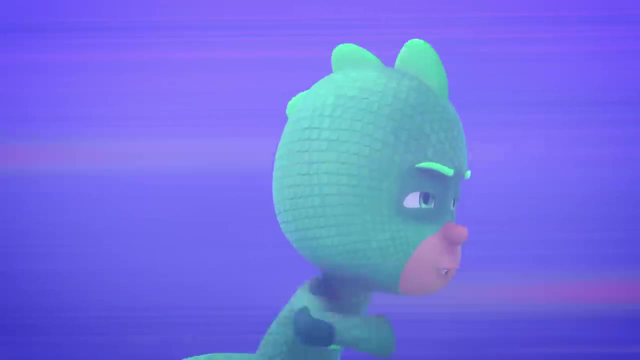 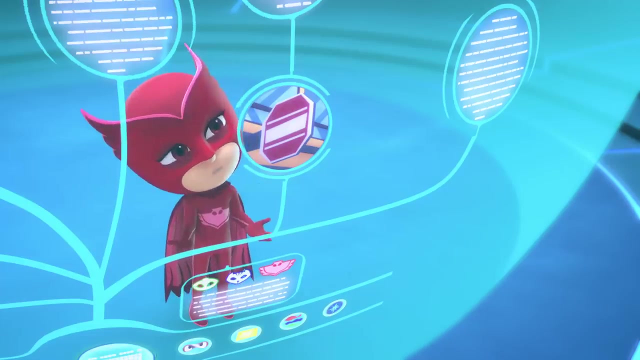 Super Gekko camouflage. Super Gekko camouflage. No way, It has sticky splat catapults. We need those things too. No, we don't, Owlette. Our base has lots of defenses already. Yeah, Owlette, think you can give us a hand out here. 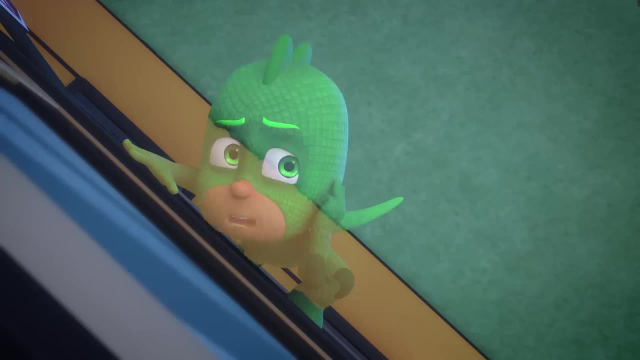 Well, I could Hello again PJ, Nink and Poops. Admit it, my headquarters is the best, And now I'm going to destroy yours. Not when we've got our own furball catapult flingers, Uh-oh. 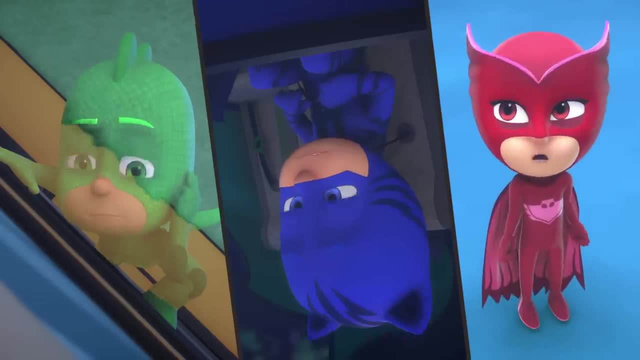 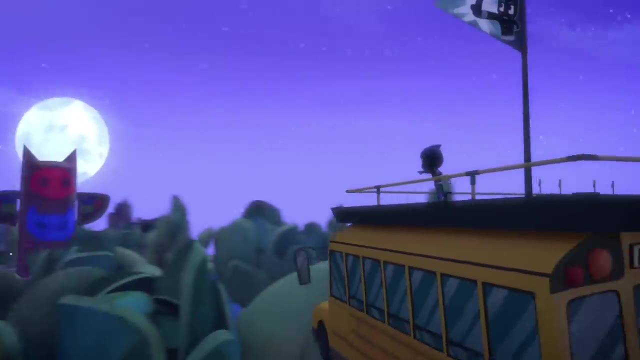 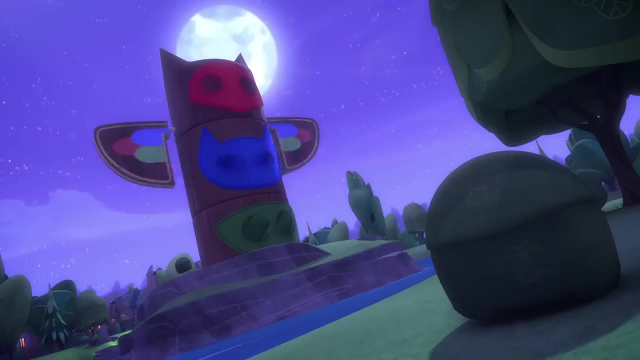 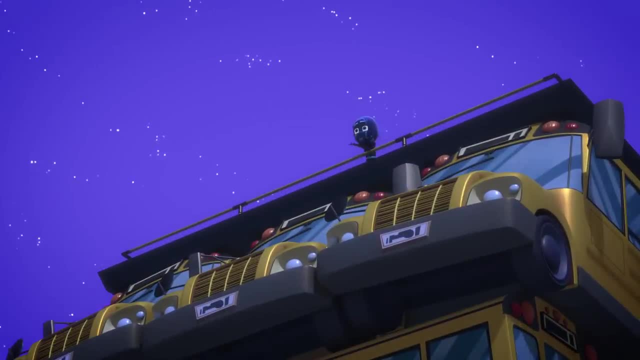 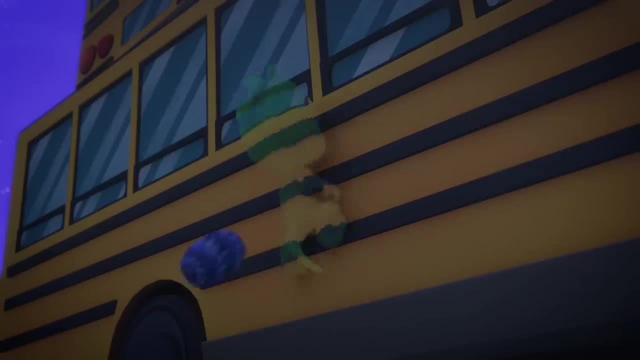 You're as blind as a bat. Just wait a minute, Owlette. You don't need to give us a hand out here. We can do this until I adjust my aim. Hey, Owlette, We're on the same team. 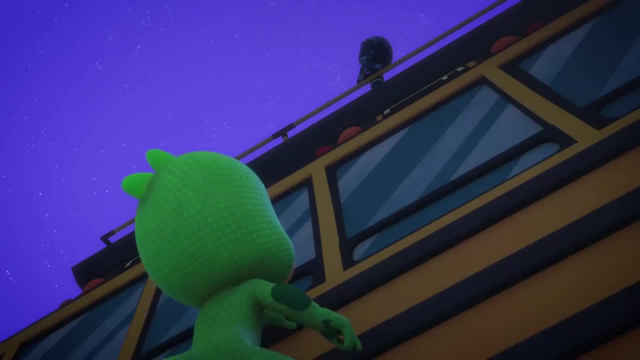 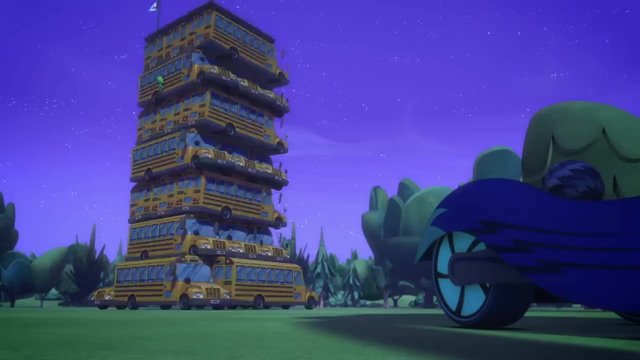 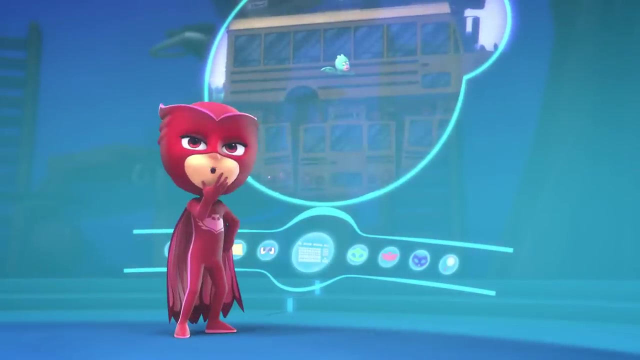 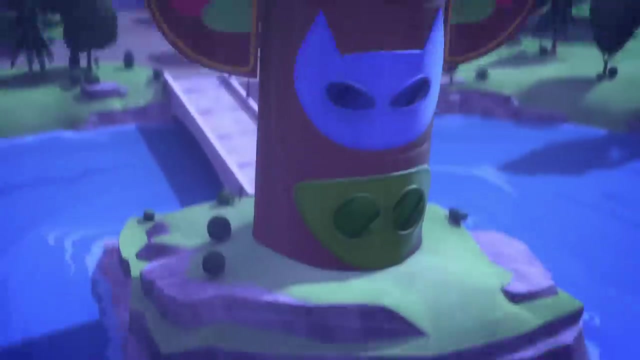 Ha, There you are, Gekko. Let me take you for a little spin. Whoa, Hold on, Gekko. Whoa, Whoa. Ah, Fluttering feathers. His fortress can spin too, Whoa. 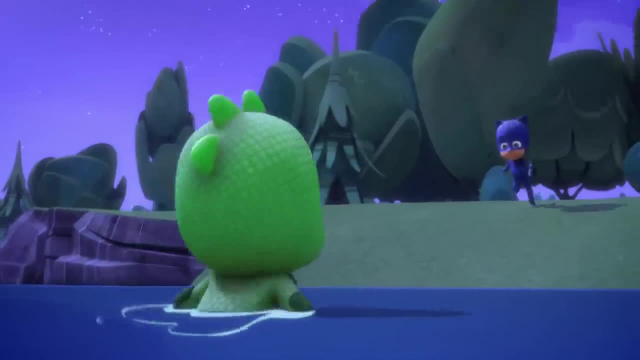 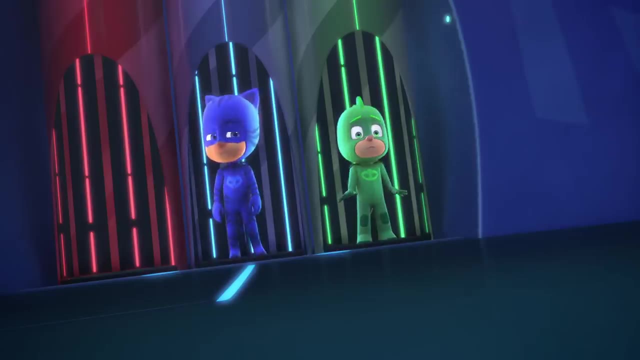 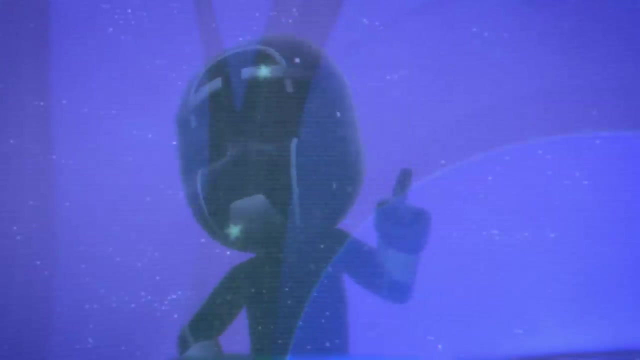 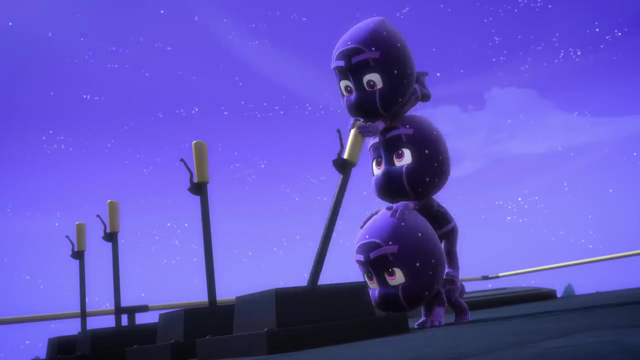 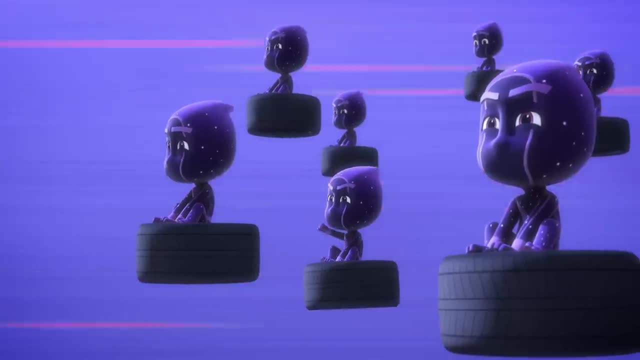 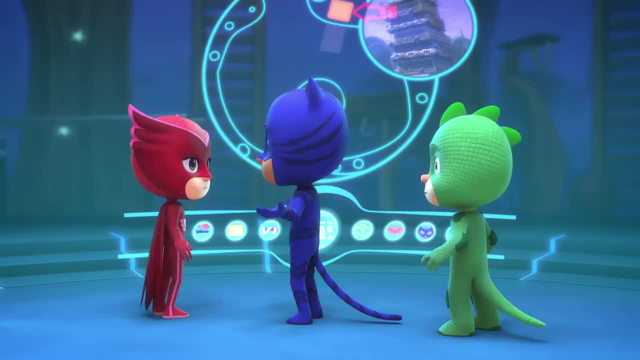 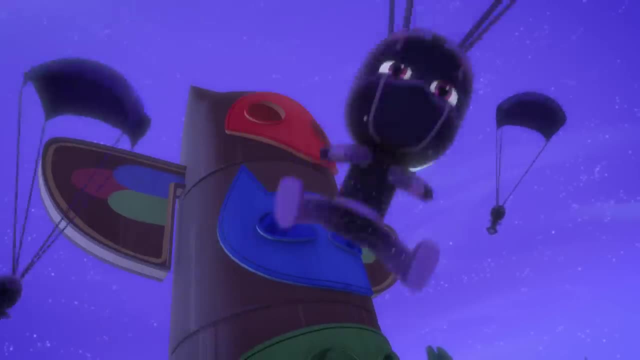 Help, Help, Help. He's filling the moat with tires, But why To make a bridge, Bringing his fortress over to destroy our base? We gotta stop him And we will By getting our base to spin just like his does. 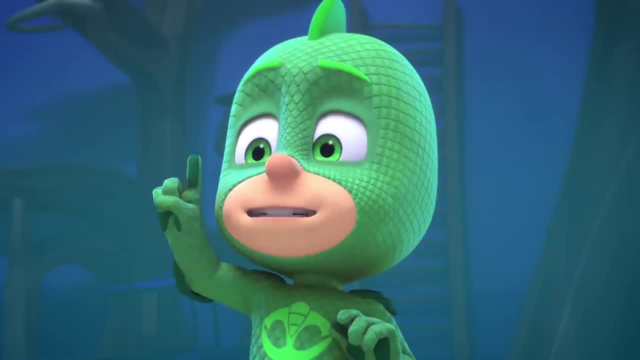 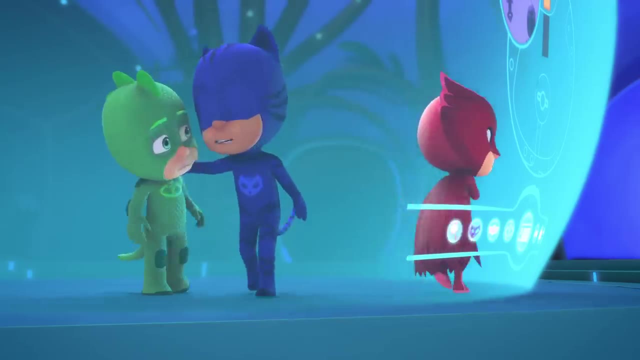 Awesome, Wait, no, Owlette, We don't need to spin. Our base has tons of great defenses already. We need to use them Right after I get the headquarters spinning. I have a plan, Gekko, I'll distract Ninjal. 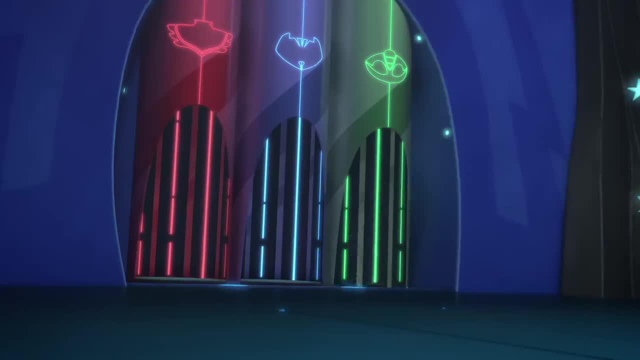 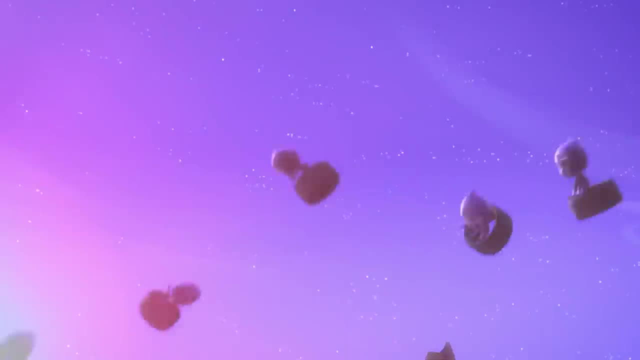 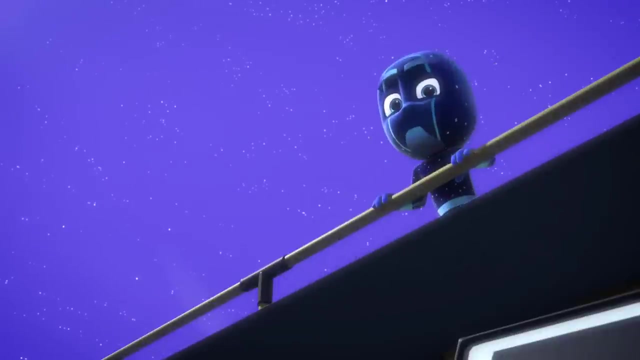 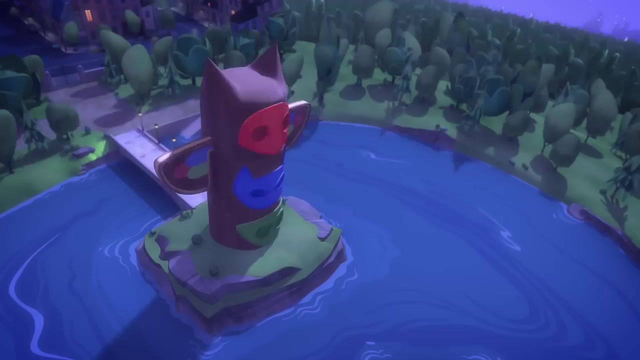 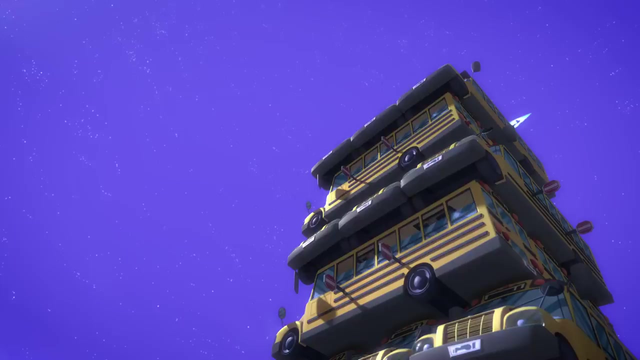 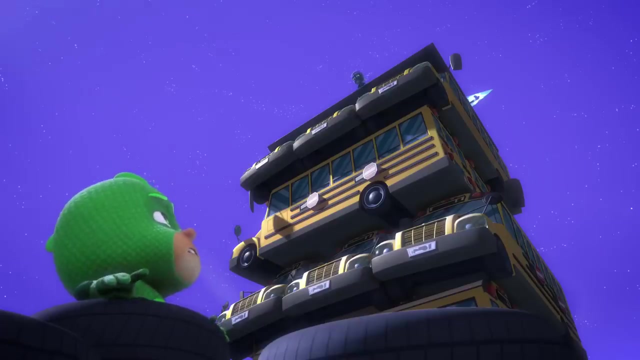 just so you can get rid of those tires, Try seeing through this. Owlbees. Aww, What Goodbye tire bridge. All right, Now we're spinning. Wait what? What, Oops, did I throw that sticky slat? 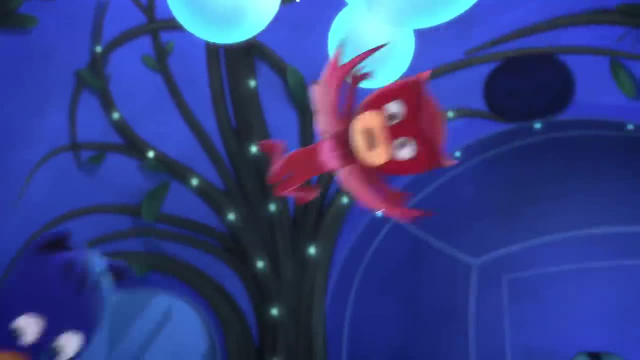 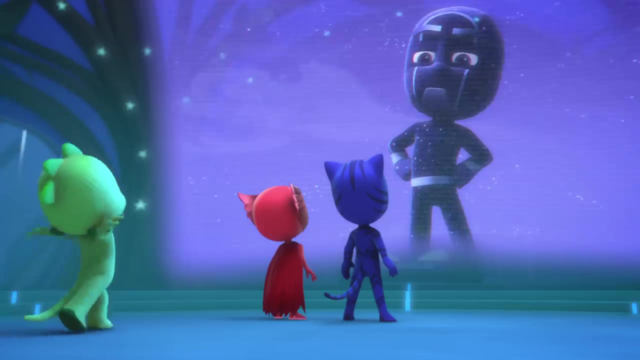 Let's do it again. Whoa, Enough playing around PJ Masks. Soon, only one fortress will be left standing. The best fortress, Mine. Oh no, Now he can cross the tire bridge. This is all my fault. Night Ninja's fortress has all these new things. 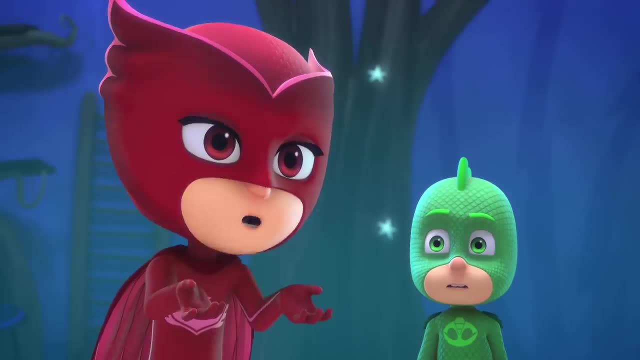 And when I saw them, I wanted them too. You guys were right. We don't need new things just because someone else has them. That's okay, Owlette, I'm sure there's something we already have that can stop him. 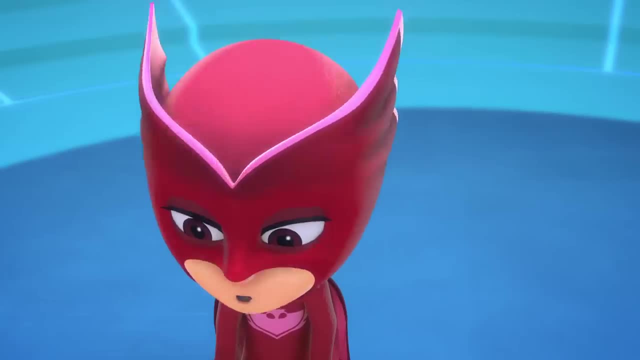 We'll get the school buses back. There is something we can use to stop him A few somethings. It's time to play a hero. Yeah, Let's go. Owlette, Owlette, Owlette, Owlette, Owlette. 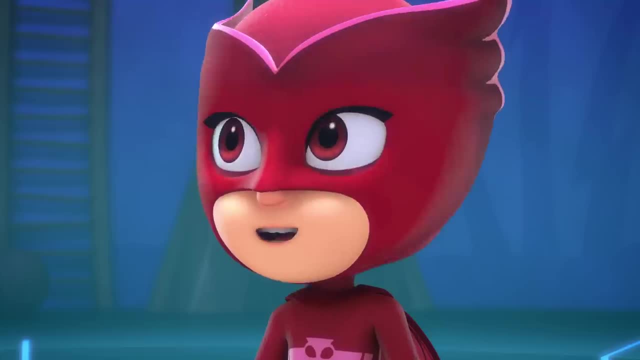 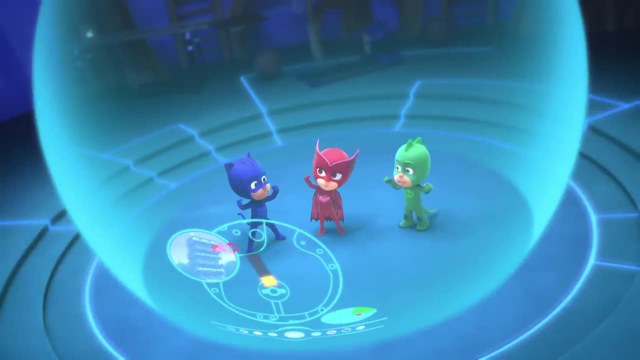 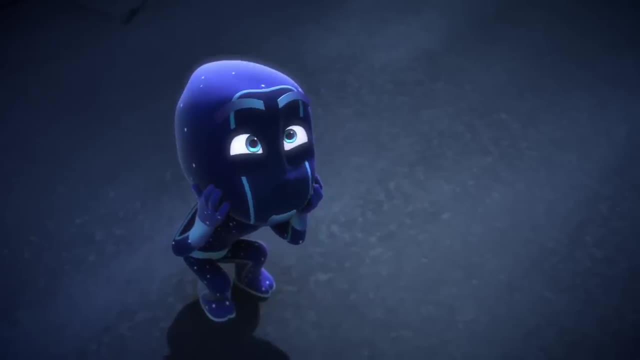 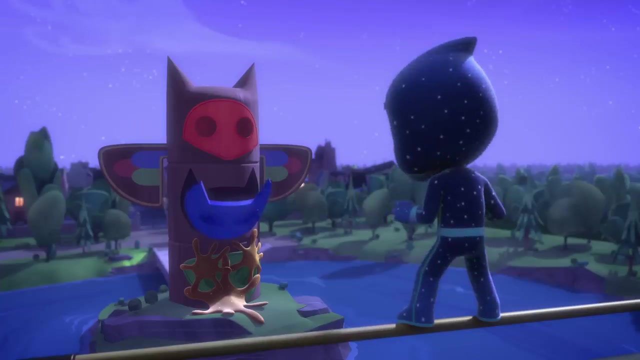 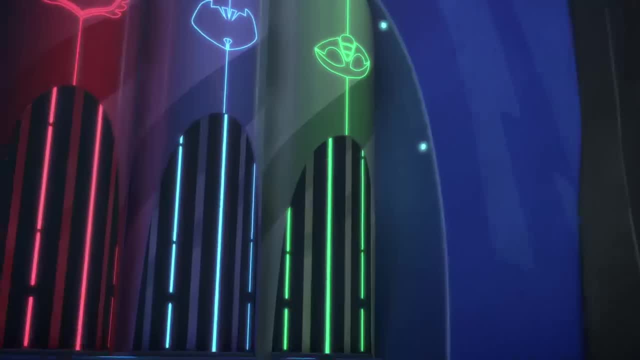 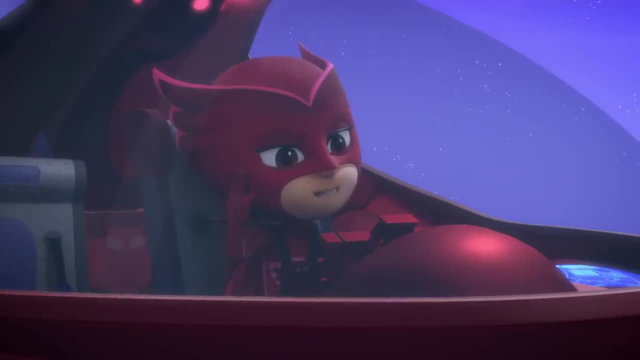 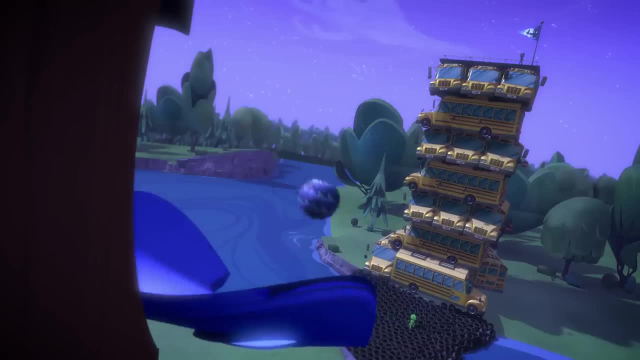 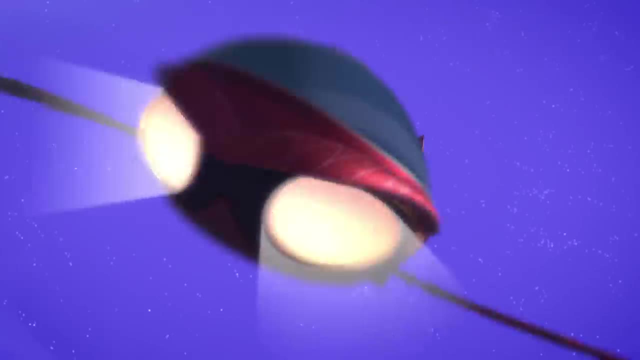 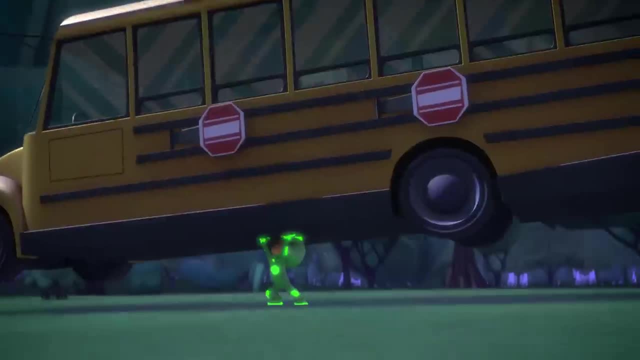 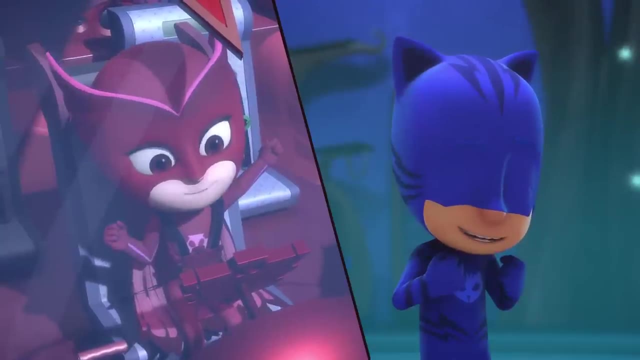 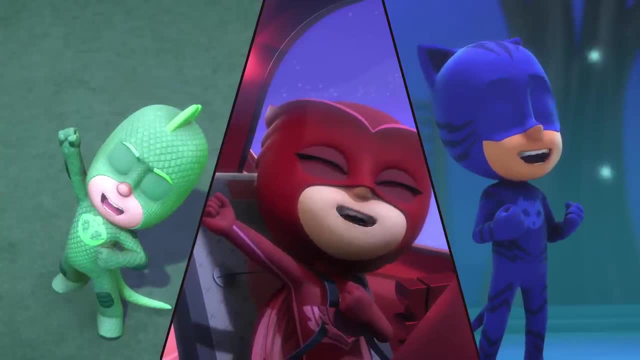 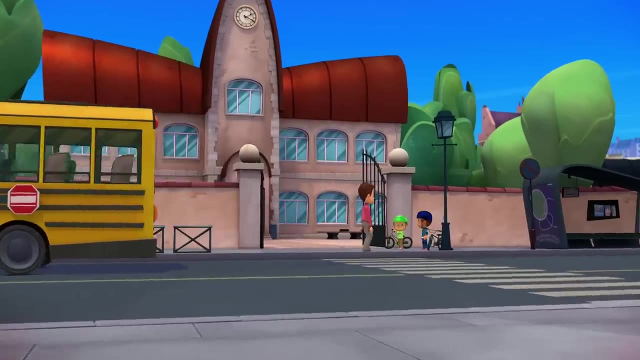 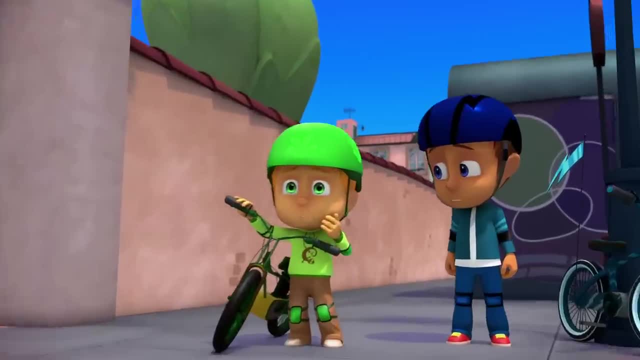 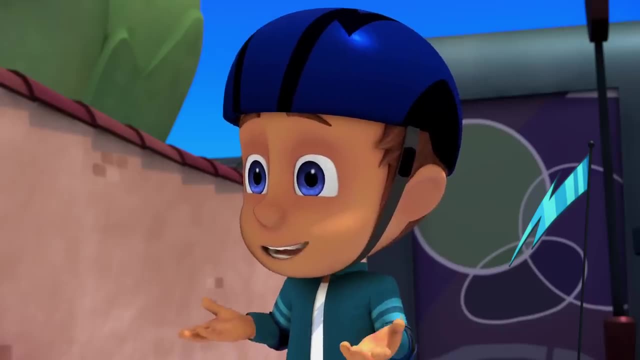 Thanks, Isn't it awesome? Oh wait, Sorry, Amaya, I didn't want to make you feel bad that you don't have a new bike. Maybe we should do something else instead. No, no, We can still go riding. 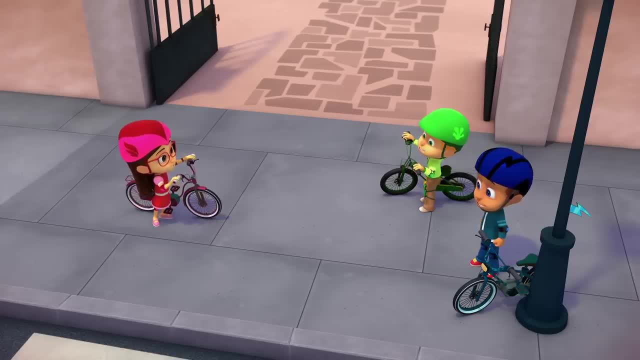 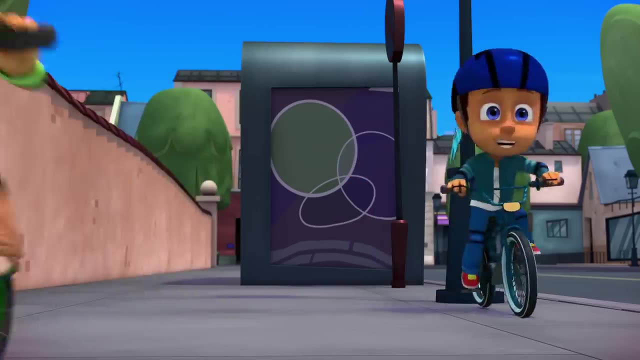 Greg's new bike is awesome, But I love my old bike too. It's still pretty great And it's fast. Catch me if you can. Bye, Bye, Bye, Bye, Bye, Bye, Bye.